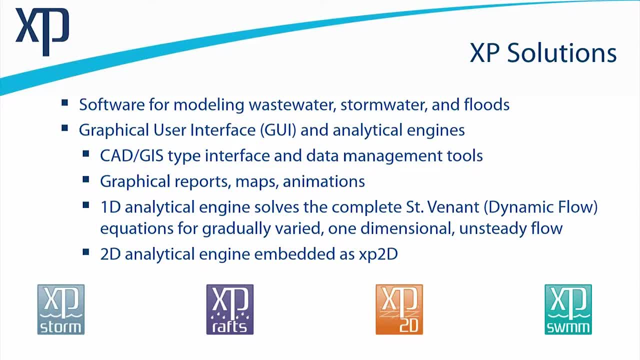 towards the end. So just briefly about XP Solutions. for those who are new to our software or if you haven't struck us in the past, XP Solutions is a software supplier and we provide solutions for waste water and storm water in particular. We have a range of products, with our dominant product being the XP Swim product, and that's. 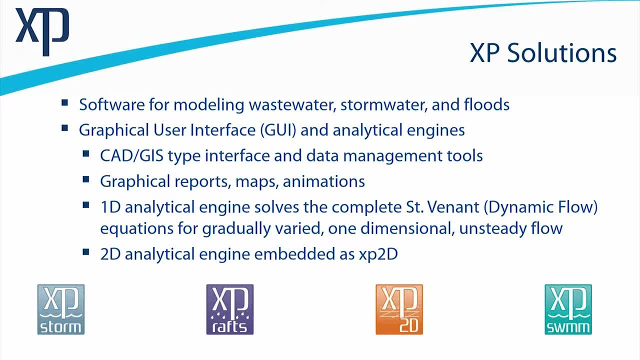 what I'm going to talk to you about today. We generate graphical user interfaces and supporting analytical engines to undertake numerical calculations. Importantly, the calculations do complete the solve, the complete segmented equations, otherwise referred to as the dynamic wave equations for gradually varied one-dimensional 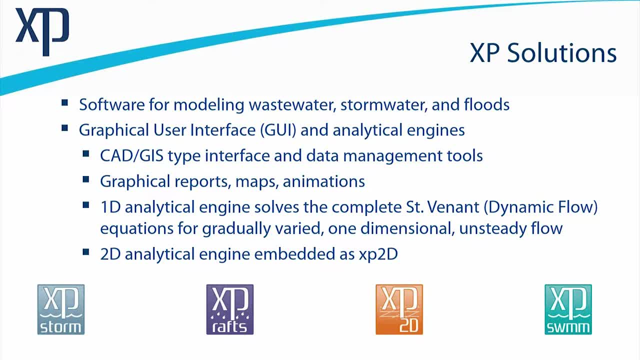 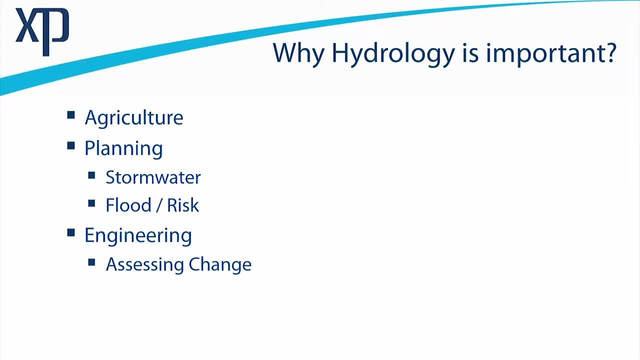 unsteady flow And we also have a two-dimensional engine, which is a module we call XP2D. So why is hydrology important? Hydrology is very important in the Malaysian context for agricultural purposes, planning purposes for development and analysing both local stormwater. 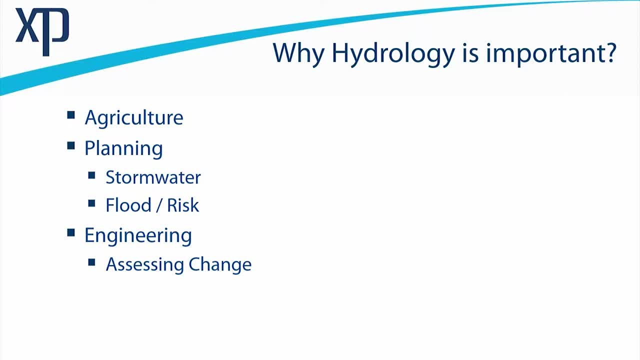 issues at a street scale and a residential scale, and also at a regional flooding and flood risk scale. From an engineering perspective, it's always about typically understanding the impact of change. What is the impact of converting an undeveloped area into a fully 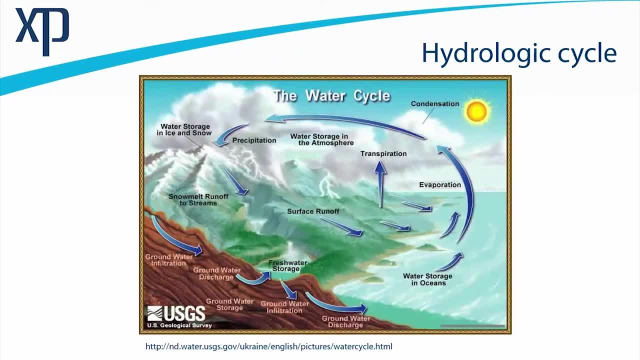 developed environment. The hydrologic cycle is obviously fundamental to hydrology, So we need to obtain our rainfall from the sky, understand how it's going to affect the environment, understand how it is conveyed along services into our storages, be they dams or river systems, discharging into groundwater or back out to the ocean or ultimate receiving. 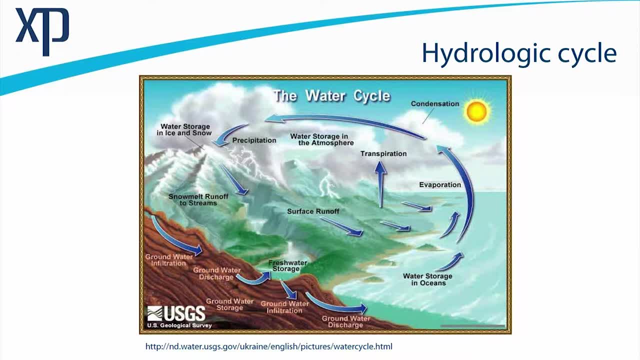 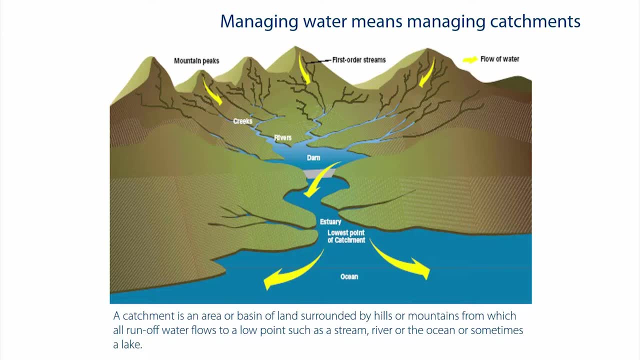 bays and the cycle starts again. From an engineering perspective, managing stormwater definitely means managing our catchments and understanding our catchments and the various contributors involved. So in the case of a high point, a high point is the first and second catchment. 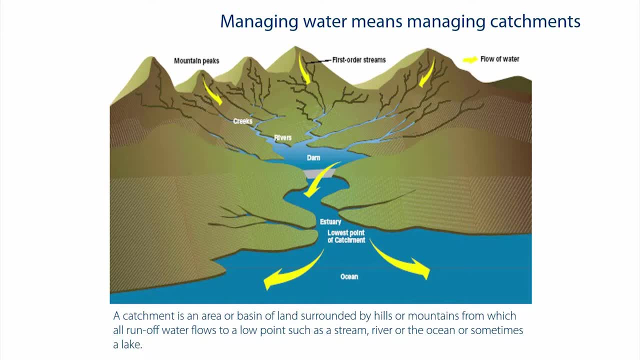 that is usually identified by the data in the national survey. The first catchment is the main catchment. the second catchment is the high point. The second catchment is the two discharges, the three discharges that are very important, But always a catchment is. 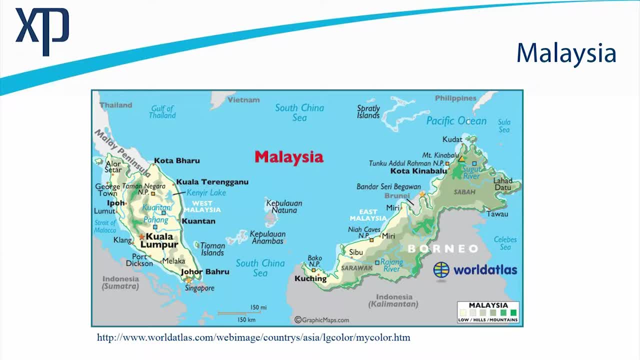 defined by ultimate high points, whether they be at a local scale or at a major geologic or topographic scale for mountain systems versus, for example, a high point in a road. Malaysia is obviously comprises of several island systems, The dominant system to the west and major areas to the east. 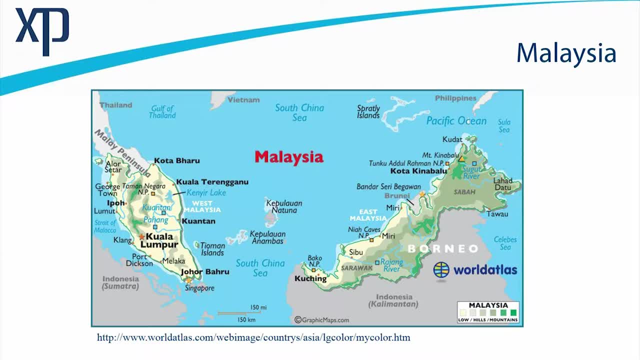 And there is key topographic elements, particularly to the west, the main areas running from Kuala Lumpur through to the north, and they define how our rainfall systems do propagate, how monsoonal systems propagate out of the South China Sea, versus the systems further to the 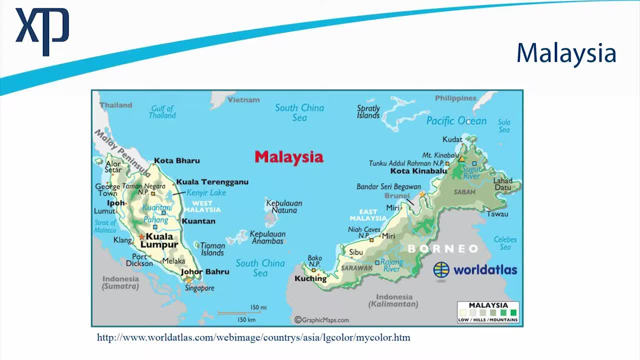 west, but also interact with systems, greater systems, even further to the east- I beg your pardon, west towards India. Now, those monsoonal systems definitely have direct impacts on when major rainfall occurs in Malaysia and how it propagates. 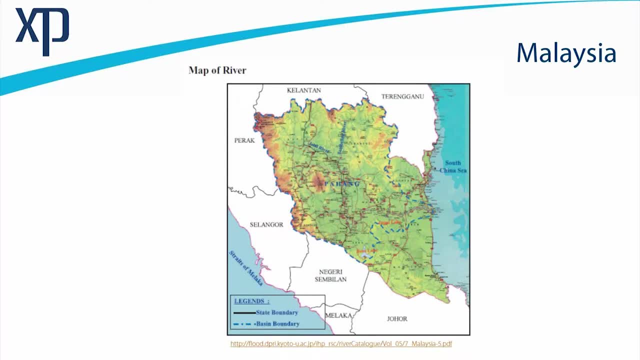 This simple map has some of the key areas, key river systems, and no doubt people listening today will have a much better appreciation of these major river systems than I do, but definitely a number of major river systems do exist. Thank you, Thank you. 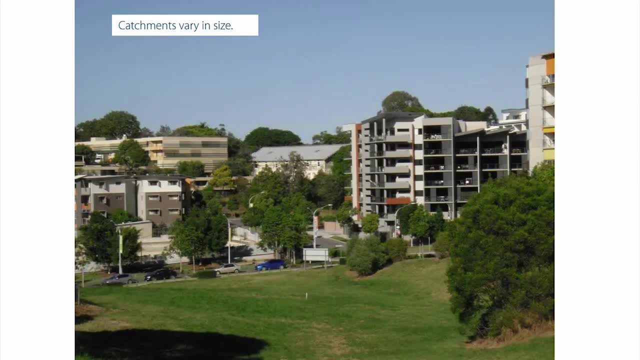 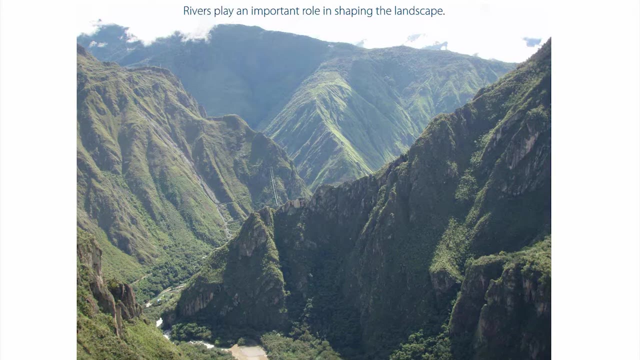 And flooding is such an important topic. Now, catchments can vary in size. They can be these local urban systems or they can be these major catchment areas, sort of as we showed on that previous slide. But rivers distinctly play an important role in shaping our landform, modifying our geographic. 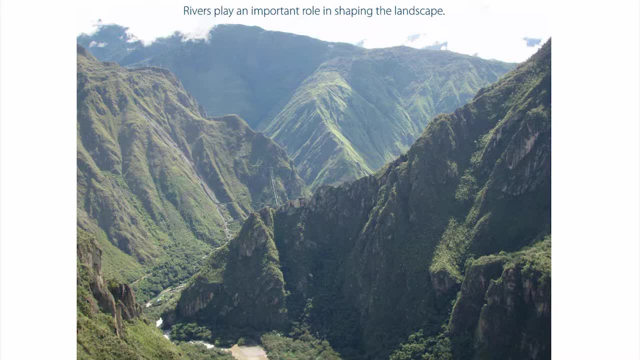 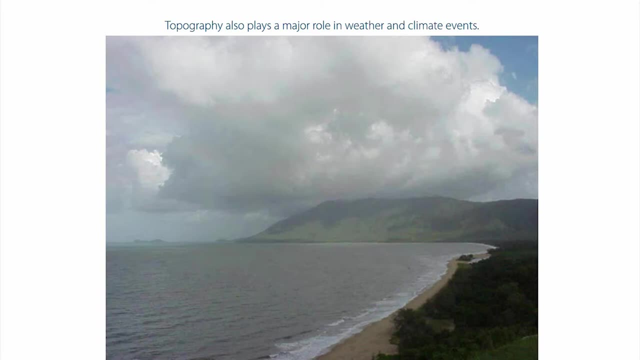 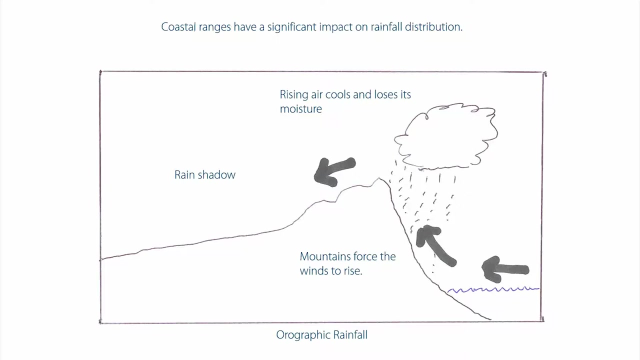 characteristics from upland areas to river downstream out to the ocean. Topography itself has a key role, as described as mountain systems that run through the centre of the western island of Malaysia has a key role in how these climatic events occur And we get systems processes such as orographic rainfall, where warm air rises, cools loses. 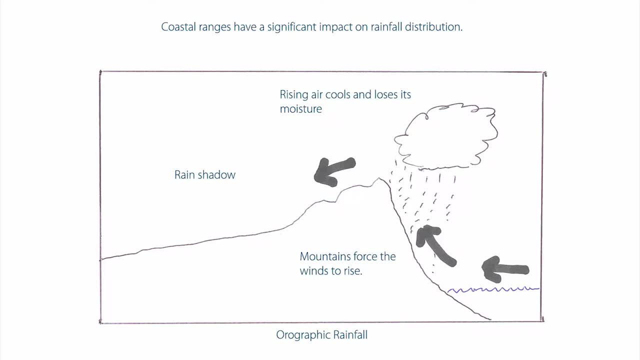 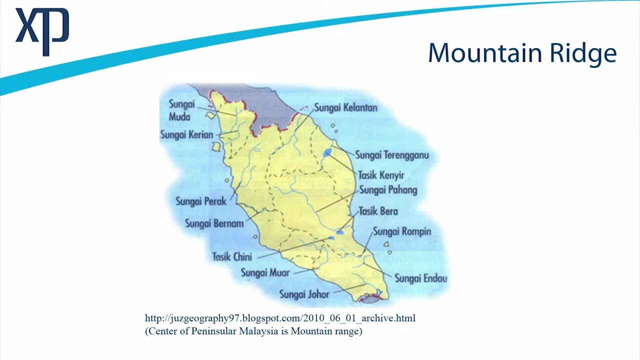 its moisture in the form of rainfall, and yet behind those mountain systems may often receive little or no rainfall at all, and that is something that can definitely occur at specific times of the year across Malaysia. And again, those mountain ridges can generally be seen here by these major river basins that 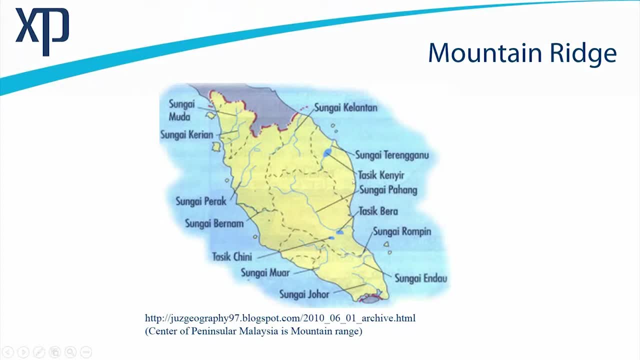 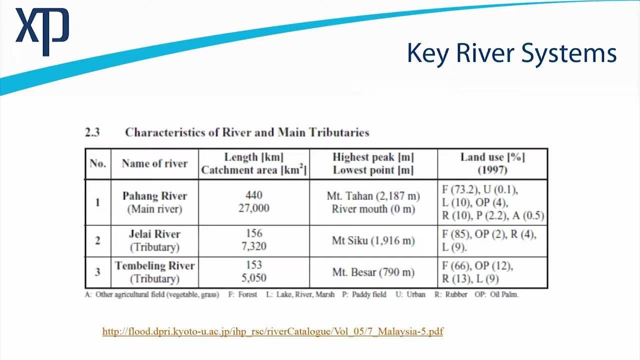 there's this distinct separation between the river basins. none of these river systems cross the eastern island. They're on the western island of Malaysia. Some general characteristics of some of the major systems can demonstrate that the length of these systems can be quite large: 440 kilometres in length for the Paying River with a catchment. 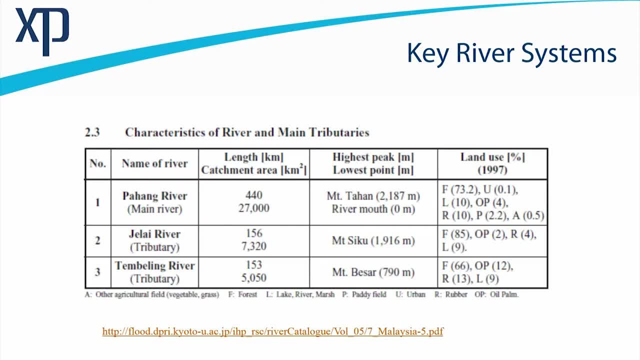 area of 27,000 square kilometres, relatively large catchment. By no means is it the Amazon or the Nile catchment, but respectively speaking it is still a relatively large system. Interestingly, it has some very high variation in topographic elevation with the top of Mount. 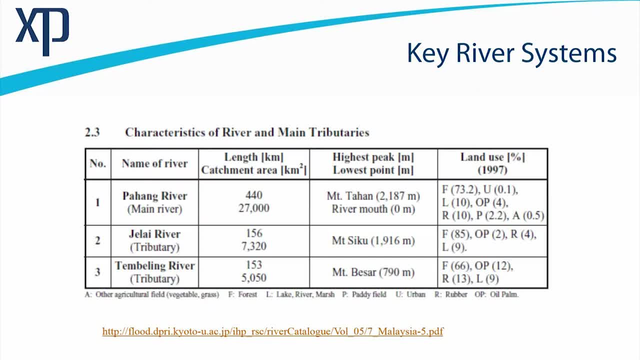 Tahan being nearly at 2,200 metres above sea level. Certainly where I am here in Australia there are very few locations that get to that elevation. There would only be one or two catchments in the entire country that would be able to have that kind of change in elevation. 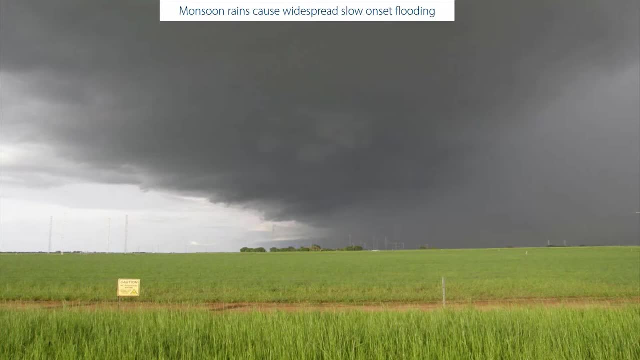 The monsoonal rain system. The monsoonal rain systems that propagate across Malaysia in the specific times of the year often cause what I'll define as slow onset flooding. It's broad in nature, broad spread, saturates catchments and can result in quite damaging. 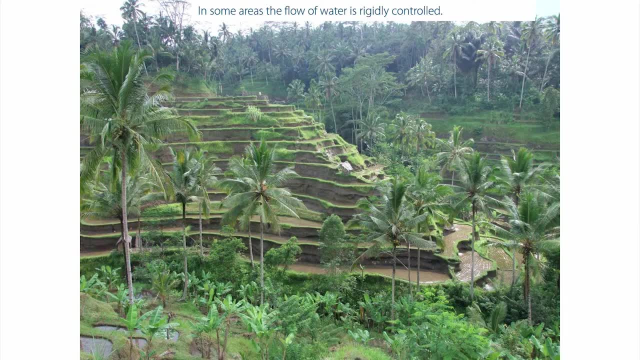 and expansive surface flooding. However, in some parts of our developed areas, for agricultural purposes, we try and hold on to and retain water, Whether that be via manual control pump systems or these defined topographic systems that can often be required. We want to try and maximise and utilise our supply of rainwater because it has such an 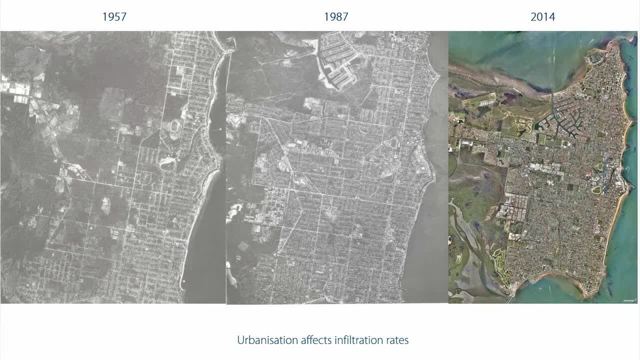 important element to our agricultural sectors. That change in hydrology too, is very important, and this three aerial photo just shows the same location over the last 60 odd years, going from limited development on the left hand side in the mid to late 1950s, development kicking in through the 1980s and some quite 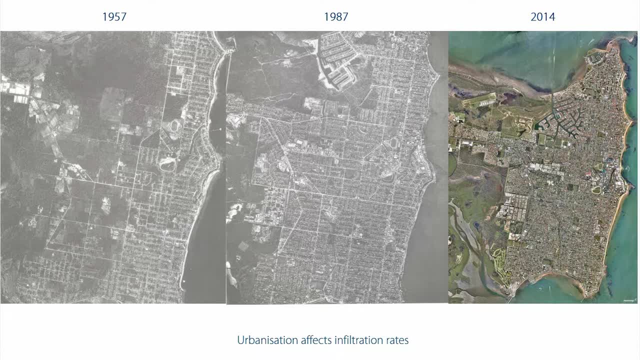 extensive development. Obviously, the photography gets better as well, as I took this from last year. This change in surface catchment details changes in particular, infiltration rates and our ability to harvest and utilise our water supplies. Final types of flooding that we can try and avoid. 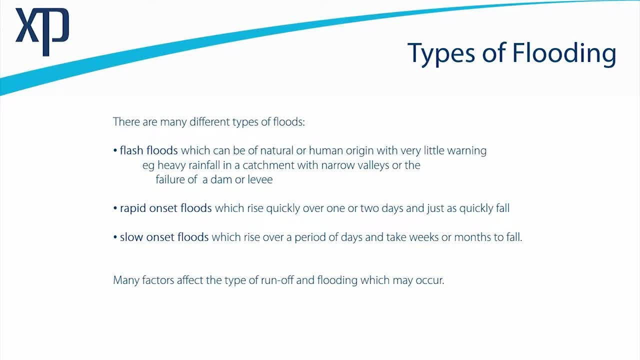 The first one is the flood We can try and observe and try and deal with from a hydrologic perspective, comprised of flash flooding, rapid onset floods and also slow onset floods, those monsoonal systems. These systems can occur either rapidly or over long periods of time and, of course, many 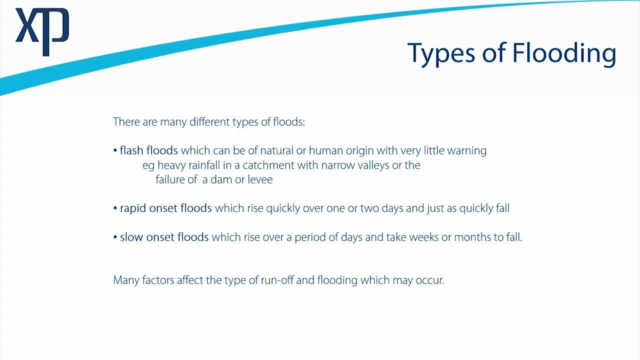 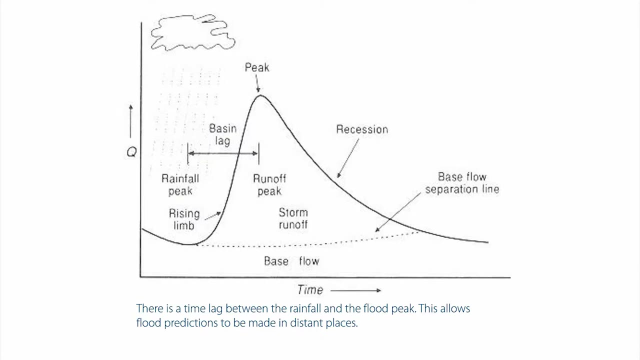 factors affect whether or not any given location is prone or subject to these three types of rainfall systems. Obviously, from a hydrology perspective, we can make these direct observations to how catchments respond to runoff, and that observation is typically made in our river systems. 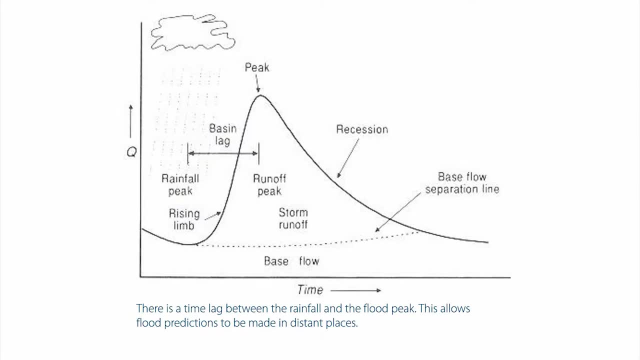 We can watch how, from the time of the rainfall occurs, what kind of lag we have until we observe our peak discharge rates and then, of course, how long it takes for that catchment to recede or dry out. Also, the interface with ongoing base flow from our groundwater systems. 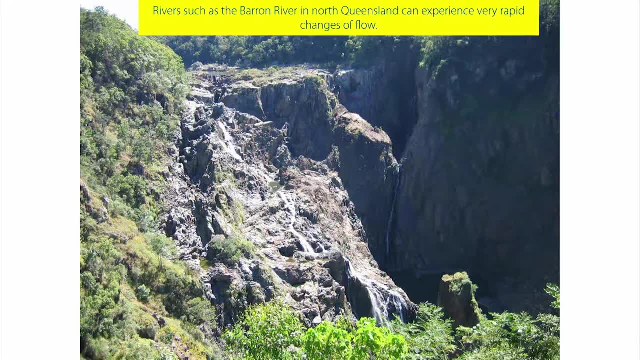 This is an example of how we can observe our peak discharge rates, and then, of course, how long it takes for that catchment to recede or dry out. Also, the interface with ongoing base flow from our groundwater systems. This is an example of how we can observe our peak discharge rates and then, of course, how 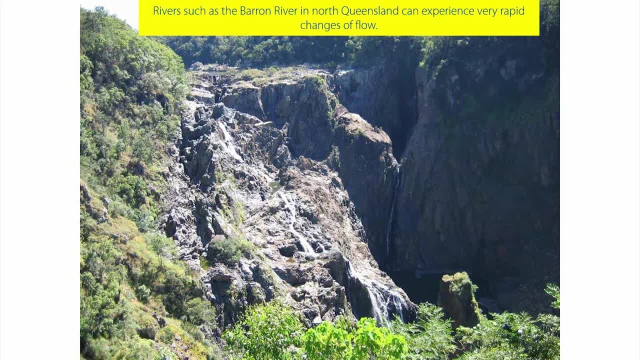 long it takes for that catchment to recede or dry out. Also, the interface with ongoing base flow from our groundwater systems. This is an example of how we can observe our peak discharge rates and then, of course, how long it takes for that catchment to recede or dry out. 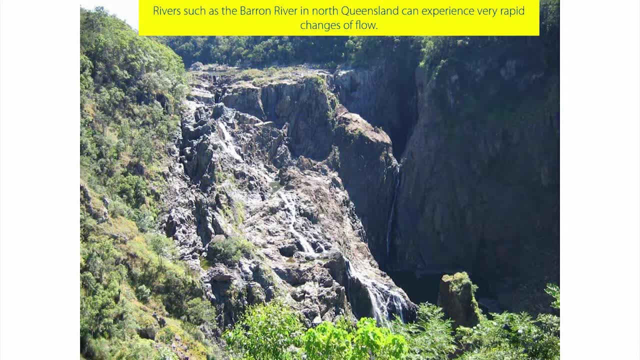 Also the interface with ongoing base flow from our groundwater systems. This is an example of how we can observe our peak discharge rates and then, of course, how long it takes for that catchment to recede or dry out. Also, the interface with ongoing base flow from our groundwater systems. 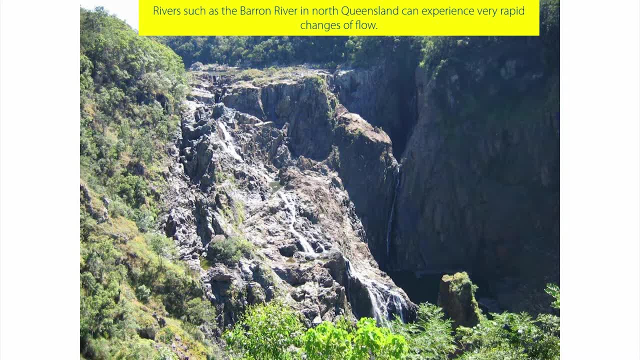 This is an example of how we can observe our peak discharge rates, and then, of course, how long it takes for that catchment to recede or dry out. Also, the interface with ongoing base flow from our groundwater systems. This is an example of how we can observe our peak discharge rates and then, of course, how 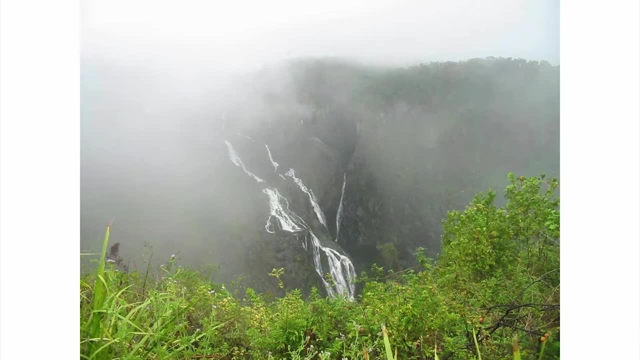 long it takes for that catchment to recede or dry out. Also, the interface with ongoing base flow from our groundwater systems. This is an example of how we can observe our peak discharge rates and then, of course, how long it takes for that catchment to recede or dry out. 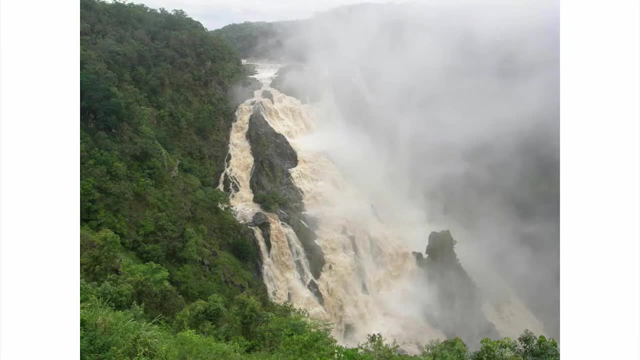 Also the interface with ongoing base flow from our groundwater systems. This is an example of how we can observe our peak discharge rates and then, of course, how long it takes for that catchment to recede or dry out. Also, the interface with ongoing base flow from our groundwater systems. 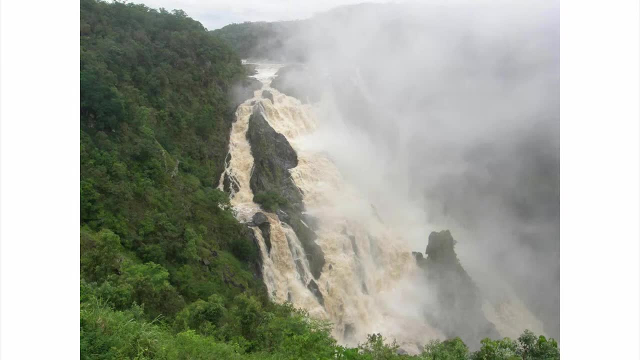 This is an example of how we can observe our peak discharge rates, and then, of course, how long it takes for that catchment to recede or dry out. Also, the interface with ongoing base flow from our groundwater systems. This is an example of how we can observe our peak discharge rates and then, of course, how 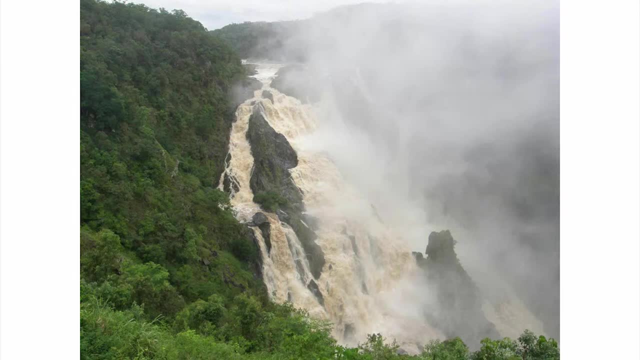 long it takes for that catchment to recede or dry out. Also, the interface with ongoing base flow from our groundwater systems. This is an example of how we can observe our peak discharge rates and then, of course, how long it takes for that catchment to recede or dry out. 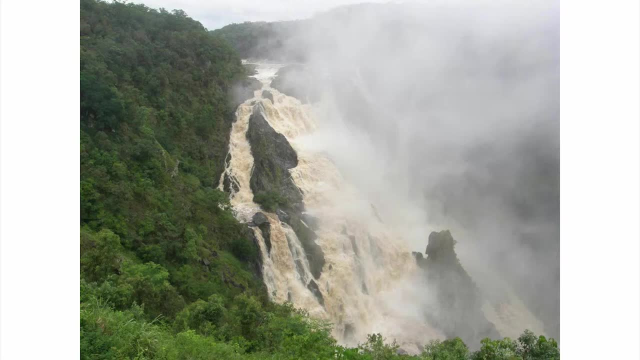 Also the interface with ongoing base flow from our groundwater systems. This is an example of how we can observe our peak discharge rates and then, of course, how long it takes for that catchment to recede or dry out. Also, the interface with ongoing base flow from our groundwater systems. 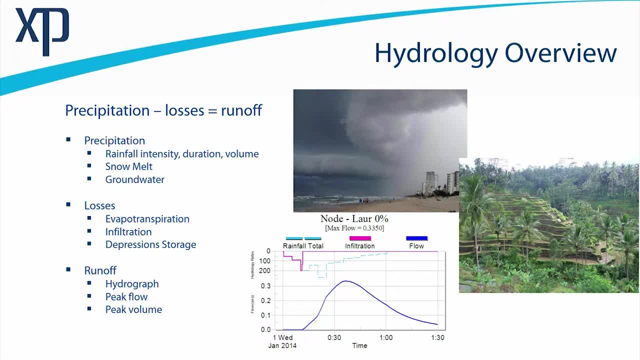 This is an example of how we can observe our peak discharge rates, and then, of course, how long it takes for that catchment to recede or dry out. Also, the interface with ongoing base flow from our groundwater systems. This is an example of how we can observe our peak discharge rates and then, of course, how 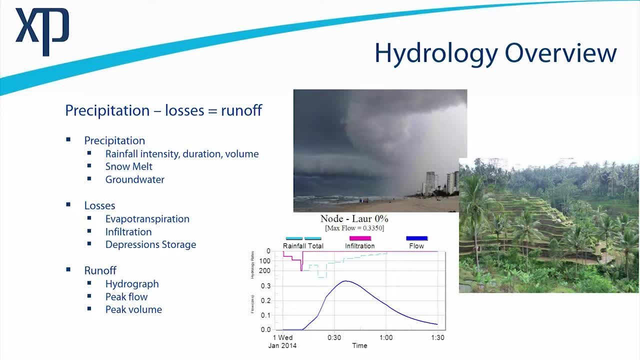 long it takes for that catchment to recede or dry out. Also, the interface with ongoing base flow from our groundwater systems. This is an example of how we can observe our peak discharge rates and then, of course, how long it takes for that catchment to recede or dry out. 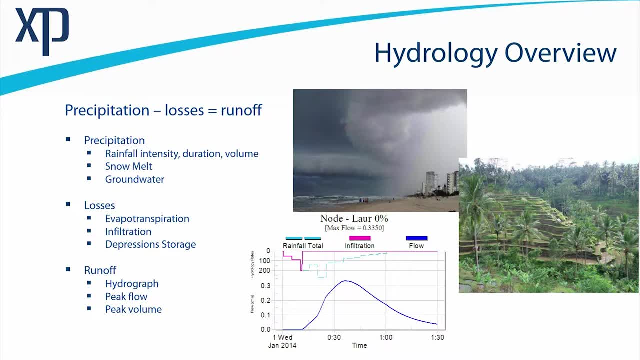 Also the interface with ongoing base flow from our groundwater systems. This is an example of how we can observe our peak discharge rates and then, of course, how long it takes for that catchment to recede or dry out. Also, the interface with ongoing base flow from our groundwater systems. 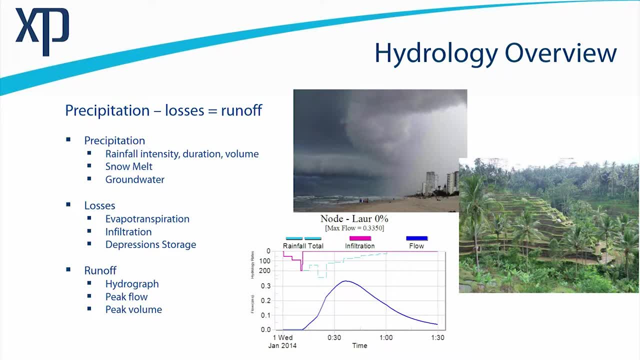 This is an example of how we can observe our peak discharge rates, and then, of course, how long it takes for that catchment to recede or dry out. Also, the interface with ongoing base flow from our groundwater systems. This is an example of how we can observe our peak discharge rates and then, of course, how 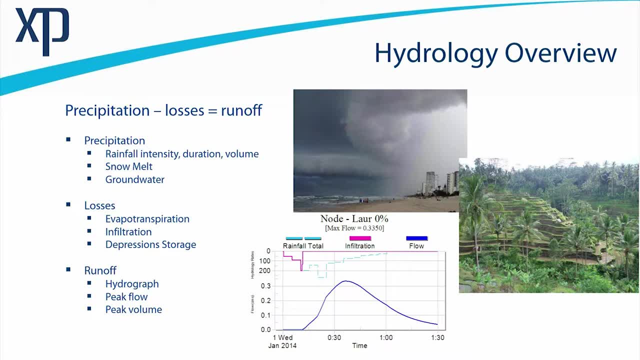 long it takes for that catchment to recede or dry out. Also, the interface with ongoing base flow from our groundwater systems. This is an example of how we can observe our peak discharge rates and then, of course, how long it takes for that catchment to recede or dry out. 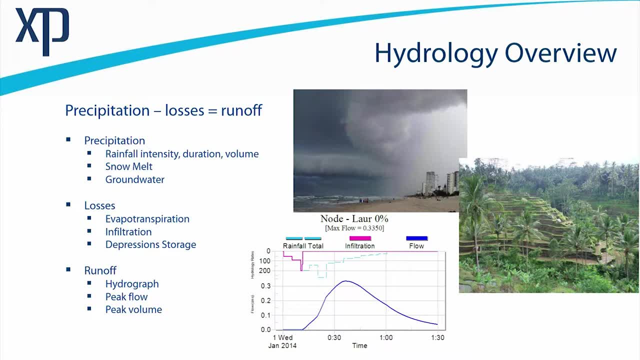 Also the interface with ongoing base flow from our groundwater systems. This is an example of how we can observe our peak discharge rates and then, of course, how long it takes for that catchment to recede or dry out. Also, the interface with ongoing base flow from our groundwater systems. 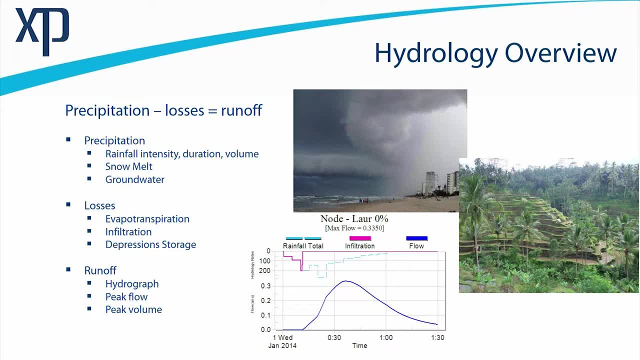 This is an example of how we can observe our peak discharge rates, and then, of course, how long it takes for that catchment to recede or dry out. Also, the interface with ongoing base flow from our groundwater systems. This is an example of how we can observe our peak discharge rates and then, of course, how 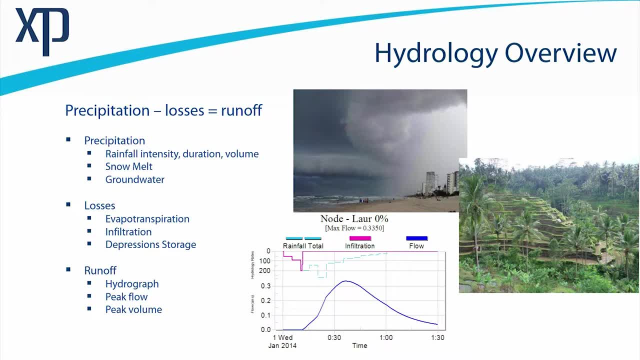 long it takes for that catchment to recede or dry out. Also, the interface with ongoing base flow from our groundwater systems. This is an example of how we can observe our peak discharge rates and then, of course, how long it takes for that catchment to recede or dry out. 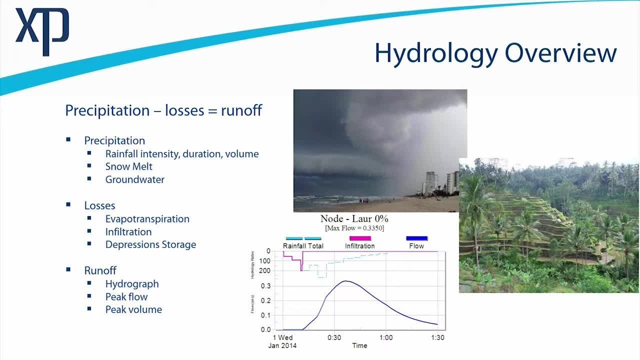 Also the interface with ongoing base flow from our groundwater systems. This is an example of how we can observe our peak discharge rates and then, of course, how long it takes for that catchment to recede or dry out. Also, the interface with ongoing base flow from our groundwater systems. 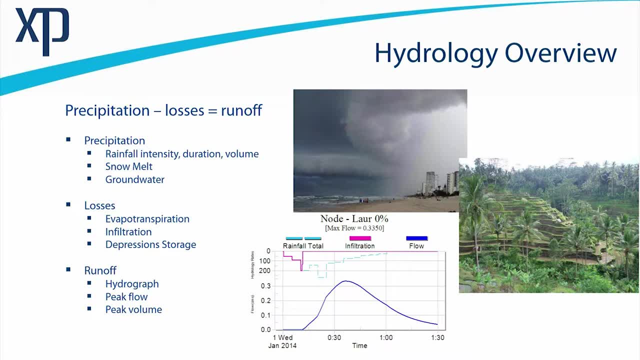 This is an example of how we can observe our peak discharge rates, and then, of course, how long it takes for that catchment to recede or dry out. Also, the interface with ongoing base flow from our groundwater systems. This is an example of how we can observe our peak discharge rates and then, of course, how 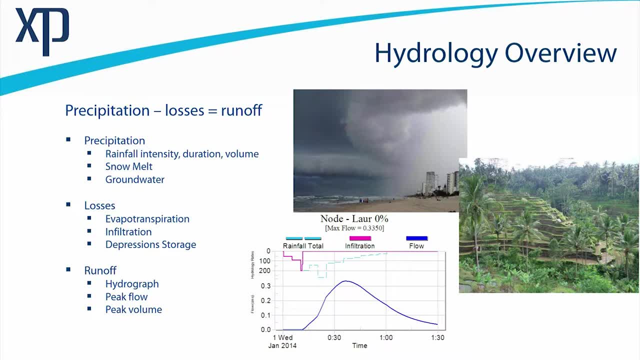 long it takes for that catchment to recede or dry out. Also, the interface with ongoing base flow from our groundwater systems. This is an example of how we can observe our peak discharge rates and then, of course, how long it takes for that catchment to recede or dry out. 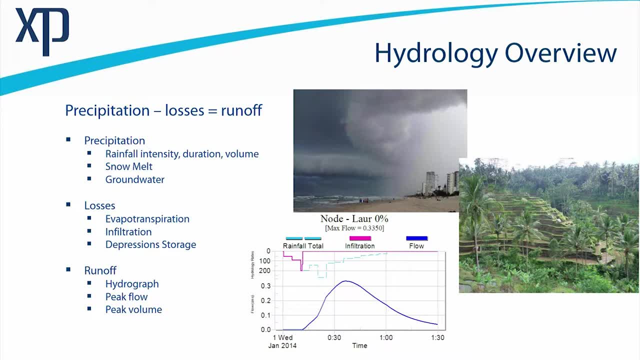 Also the interface with ongoing base flow from our groundwater systems. This is an example of how we can observe our peak discharge rates and then, of course, how long it takes for that catchment to recede or dry out. Also, the interface with ongoing base flow from our groundwater systems. 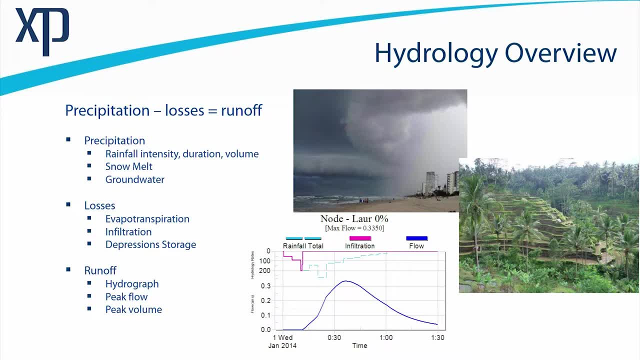 This is an example of how we can observe our peak discharge rates, and then, of course, how long it takes for that catchment to recede or dry out. Also, the interface with ongoing base flow from our groundwater systems. This is an example of how we can observe our peak discharge rates and then, of course, how 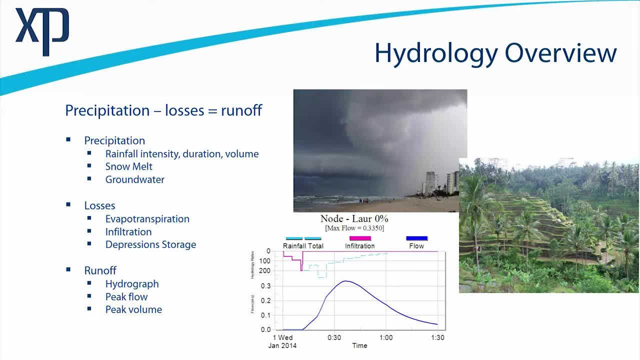 long it takes for that catchment to recede or dry out. Also, the interface with ongoing base flow from our groundwater systems. This is an example of how we can observe our peak discharge rates and then, of course, how long it takes for that catchment to recede or dry out. 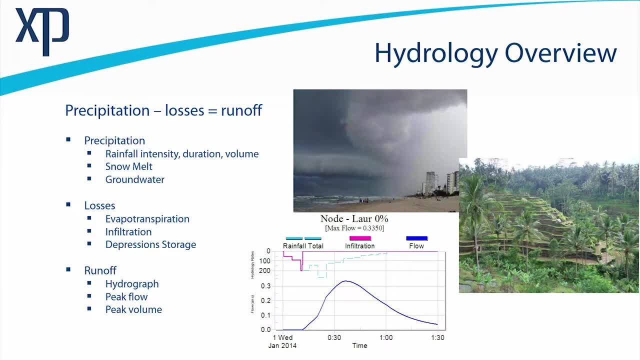 Also the interface with ongoing base flow from our groundwater systems. This is an example of how we can observe our peak discharge rates and then, of course, how long it takes for that catchment to recede or dry out. Also, the interface with ongoing base flow from our groundwater systems. 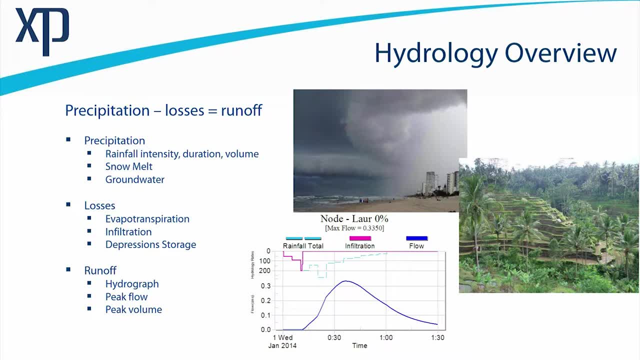 This is an example of how we can observe our peak discharge rates, and then, of course, how long it takes for that catchment to recede or dry out. Also, the interface with ongoing base flow from our groundwater systems. This is an example of how we can observe our peak discharge rates and then, of course, how 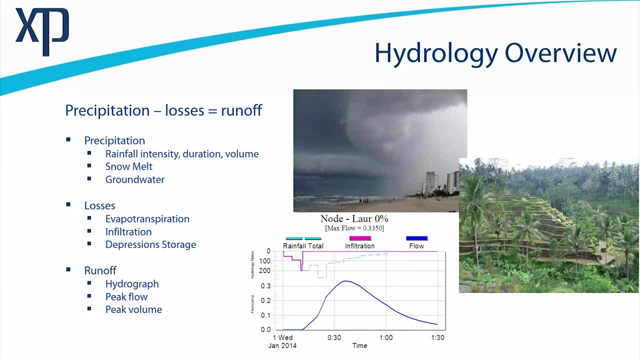 long it takes for that catchment to recede or dry out. Also, the interface with ongoing base flow from our groundwater systems. This is an example of how we can observe our peak discharge rates and then, of course, how long it takes for that catchment to recede or dry out. 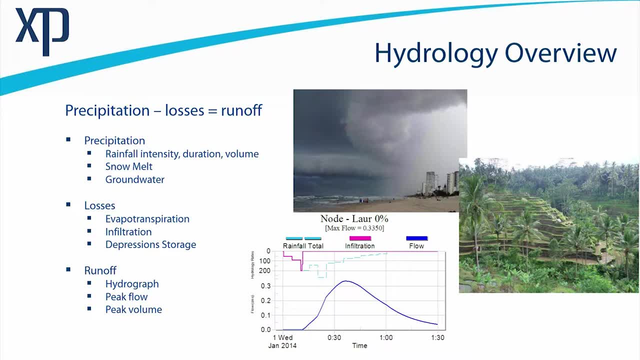 Also the interface with ongoing base flow from our groundwater systems. This is an example of how we can observe our peak discharge rates and then, of course, how long it takes for that catchment to recede or dry out. Also, the interface with ongoing base flow from our groundwater systems. 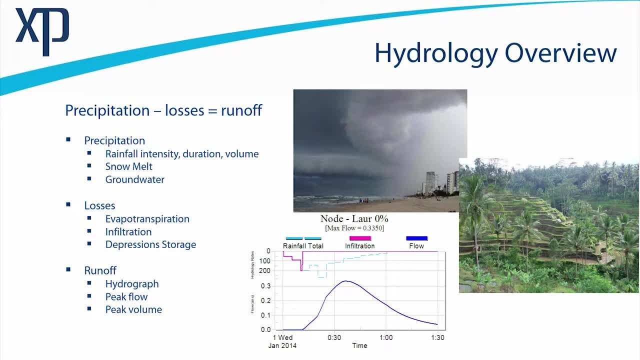 This is an example of how we can observe our peak discharge rates, and then, of course, how long it takes for that catchment to recede or dry out. Also, the interface with ongoing base flow from our groundwater systems. This is an example of how we can observe our peak discharge rates and then, of course, how 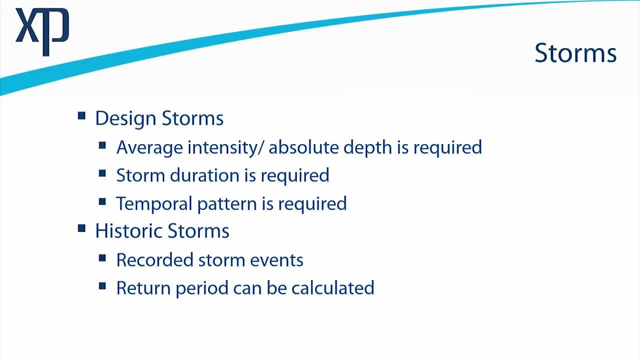 long it takes for that catchment to recede or dry out. Also, the interface with ongoing base flow from our groundwater systems. This is an example of how we can observe our peak discharge rates and then, of course, how long it takes for that catchment to recede or dry out. 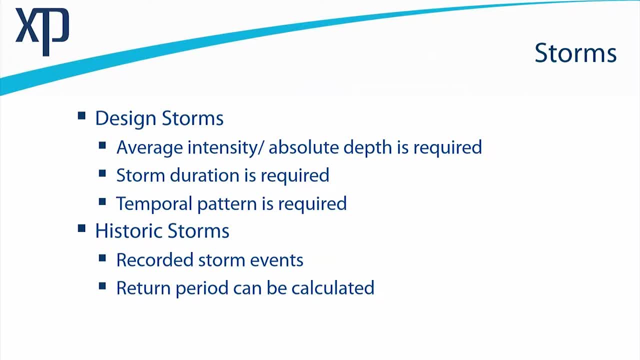 Also the interface with ongoing base flow from our groundwater systems. This is an example of how we can observe our peak discharge rates and then, of course, how long it takes for that catchment to recede or dry out. Also, the interface with ongoing base flow from our groundwater systems. 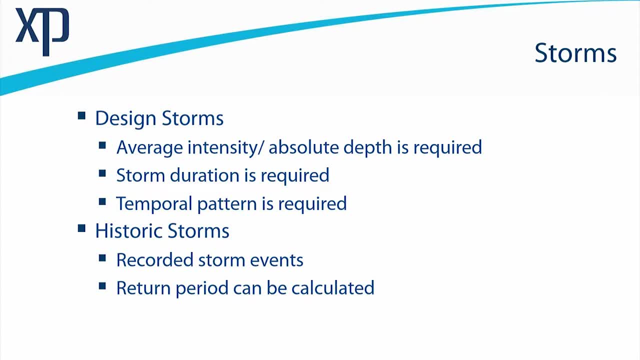 This is an example of how we can observe our peak discharge rates, and then, of course, how long it takes for that catchment to recede or dry out. Also, the interface with ongoing base flow from our groundwater systems. This is an example of how we can observe our peak discharge rates and then, of course, how 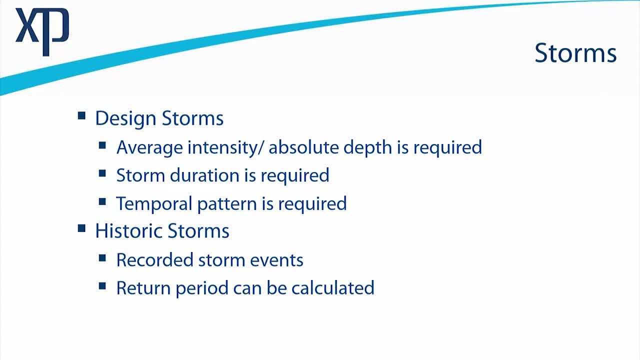 long it takes for that catchment to recede or dry out. Also, the interface with ongoing base flow from our groundwater systems. This is an example of how we can observe our peak discharge rates and then, of course, how long it takes for that catchment to recede or dry out. 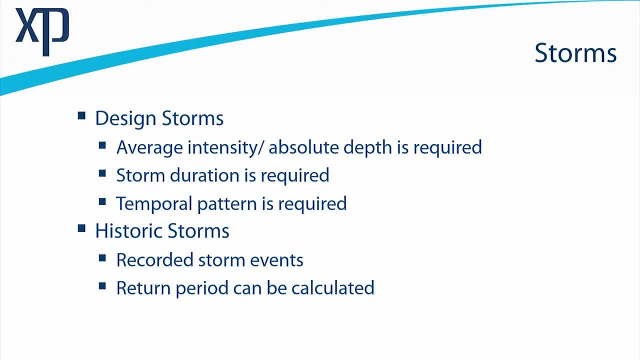 Also the interface with ongoing base flow from our groundwater systems. This is an example of how we can observe our peak discharge rates and then, of course, how long it takes for that catchment to recede or dry out. Also, the interface with ongoing base flow from our groundwater systems. 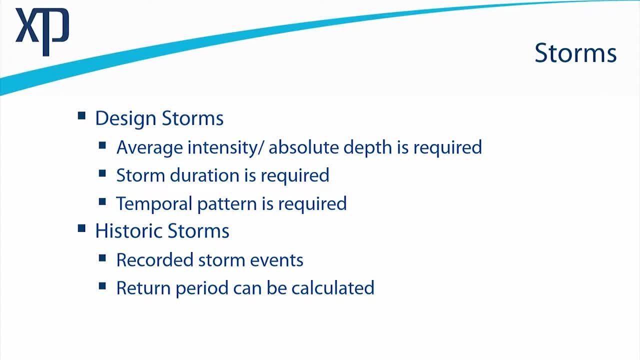 This is an example of how we can observe our peak discharge rates, and then, of course, how long it takes for that catchment to recede or dry out. Also, the interface with ongoing base flow from our groundwater systems. This is an example of how we can observe our peak discharge rates and then, of course, how 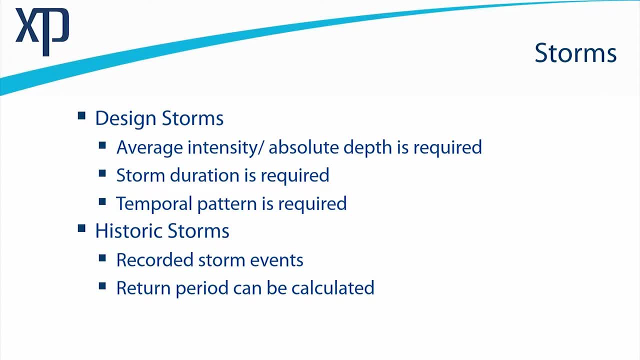 long it takes for that catchment to recede or dry out. Also, the interface with ongoing base flow from our groundwater systems. This is an example of how we can observe our peak discharge rates and then, of course, how long it takes for that catchment to recede or dry out. 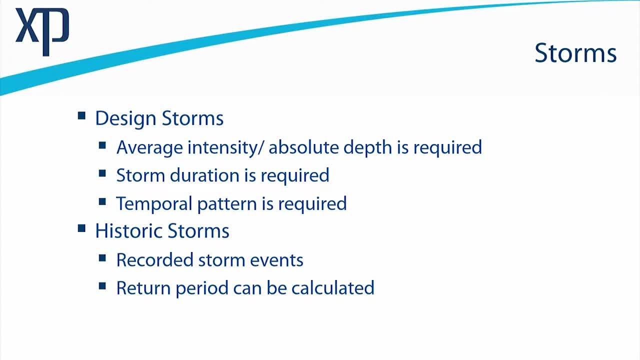 Also the interface with ongoing base flow from our groundwater systems. This is an example of how we can observe our peak discharge rates and then, of course, how long it takes for that catchment to recede or dry out. Also, the interface with ongoing base flow from our groundwater systems. 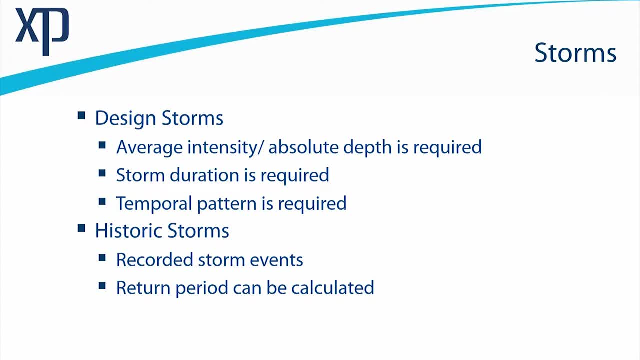 This is an example of how we can observe our peak discharge rates, and then, of course, how long it takes for that catchment to recede or dry out. Also, the interface with ongoing base flow from our groundwater systems. This is an example of how we can observe our peak discharge rates and then, of course, how 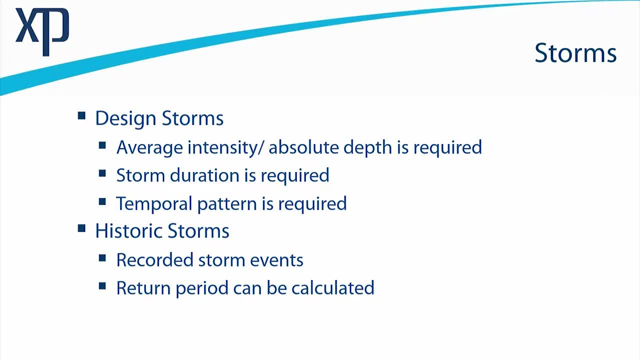 long it takes for that catchment to recede or dry out. Also, the interface with ongoing base flow from our groundwater systems. This is an example of how we can observe our peak discharge rates and then, of course, how long it takes for that catchment to recede or dry out. 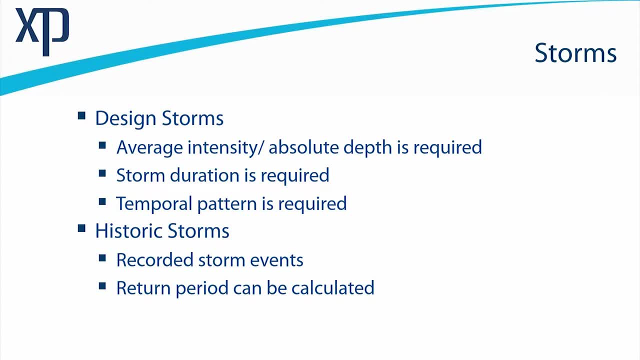 Also the interface with ongoing base flow from our groundwater systems. This is an example of how we can observe our peak discharge rates and then, of course, how long it takes for that catchment to recede or dry out. Also, the interface with ongoing base flow from our groundwater systems. 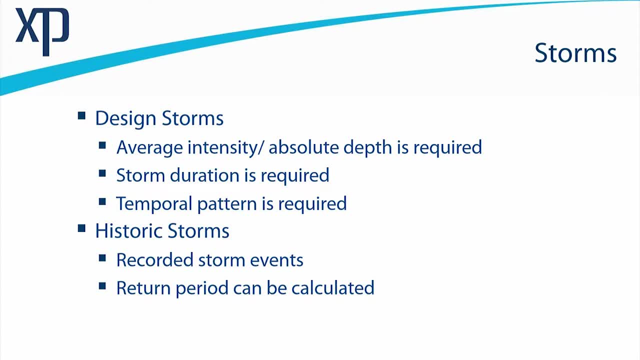 This is an example of how we can observe our peak discharge rates, and then, of course, how long it takes for that catchment to recede or dry out. Also, the interface with ongoing base flow from our groundwater systems. This is an example of how we can observe our peak discharge rates and then, of course, how 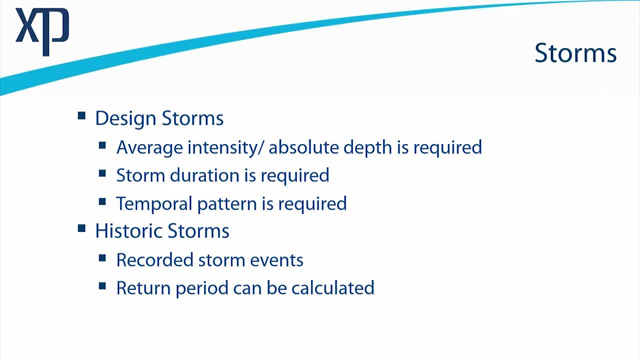 long it takes for that catchment to recede or dry out. Also, the interface with ongoing base flow from our groundwater systems. This is an example of how we can observe our peak discharge rates and then, of course, how long it takes for that catchment to recede or dry out. 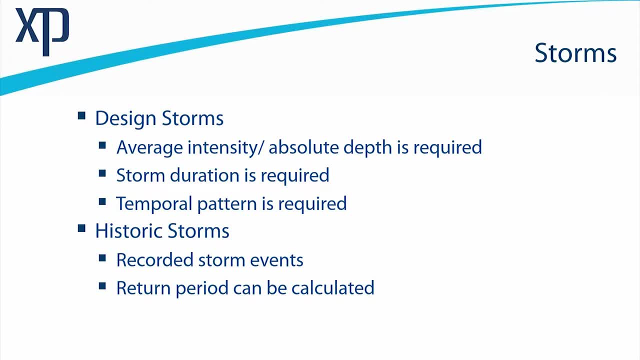 Also the interface with ongoing base flow from our groundwater systems. This is an example of how we can observe our peak discharge rates and then, of course, how long it takes for that catchment to recede or dry out. Also, the interface with ongoing base flow from our groundwater systems. 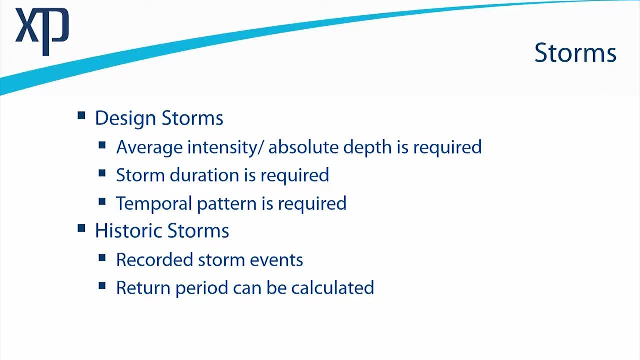 This is an example of how we can observe our peak discharge rates, and then, of course, how long it takes for that catchment to recede or dry out. Also, the interface with ongoing base flow from our groundwater systems. This is an example of how we can observe our peak discharge rates and then, of course, how 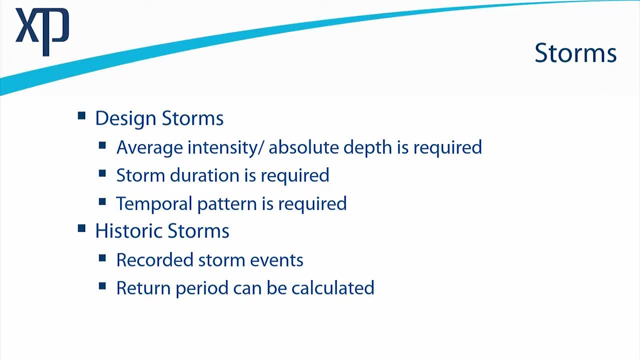 long it takes for that catchment to recede or dry out. Also, the interface with ongoing base flow from our groundwater systems. This is an example of how we can observe our peak discharge rates and then, of course, how long it takes for that catchment to recede or dry out. 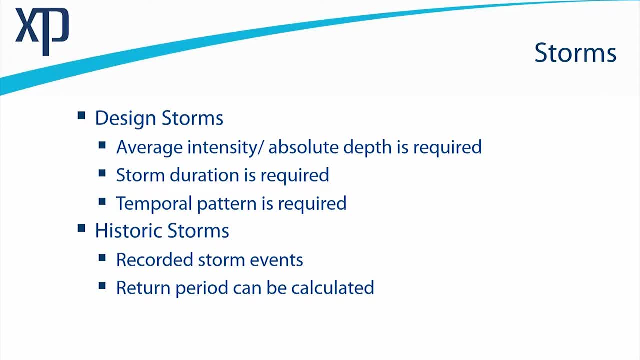 Also the interface with ongoing base flow from our groundwater systems. This is an example of how we can observe our peak discharge rates and then, of course, how long it takes for that catchment to recede or dry out. Also, the interface with ongoing base flow from our groundwater systems. 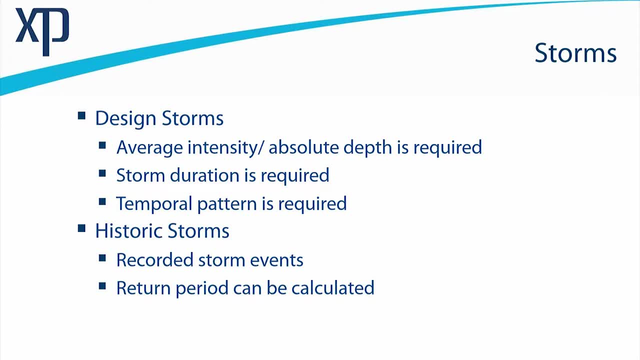 This is an example of how we can observe our peak discharge rates, and then, of course, how long it takes for that catchment to recede or dry out. Also, the interface with ongoing base flow from our groundwater systems. This is an example of how we can observe our peak discharge rates and then, of course, how 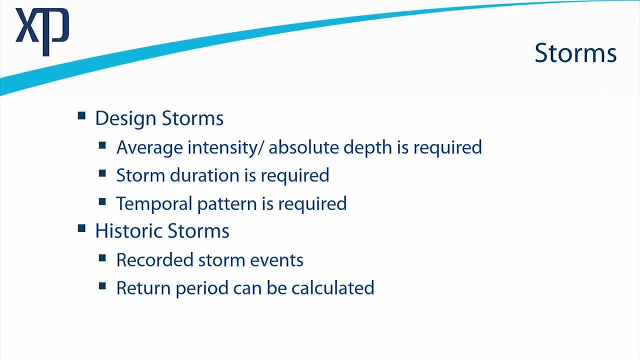 long it takes for that catchment to recede or dry out. Also, the interface with ongoing base flow from our groundwater systems. This is an example of how we can observe our peak discharge rates and then, of course, how long it takes for that catchment to recede or dry out. 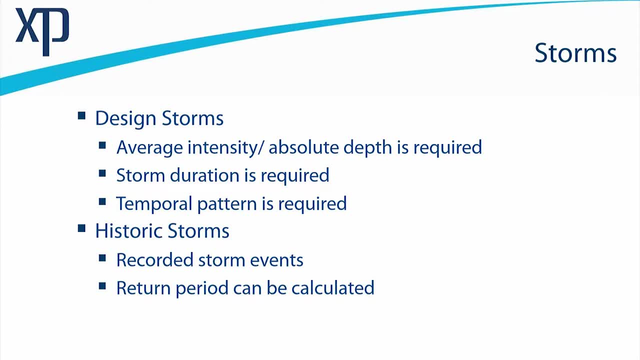 Also the interface with ongoing base flow from our groundwater systems. This is an example of how we can observe our peak discharge rates and then, of course, how long it takes for that catchment to recede or dry out. Also, the interface with ongoing base flow from our groundwater systems. 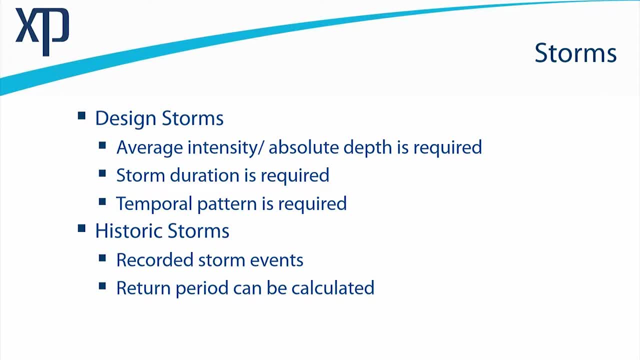 This is an example of how we can observe our peak discharge rates, and then, of course, how long it takes for that catchment to recede or dry out. Also, the interface with ongoing base flow from our groundwater systems. This is an example of how we can observe our peak discharge rates and then, of course, how 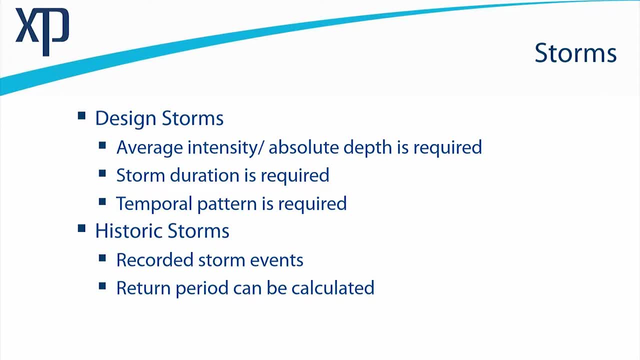 long it takes for that catchment to recede or dry out. Also, the interface with ongoing base flow from our groundwater systems And for the Malaysian region, which is our intensity frequency calculator, it's a very useful tool to get you quickly into your modelling. 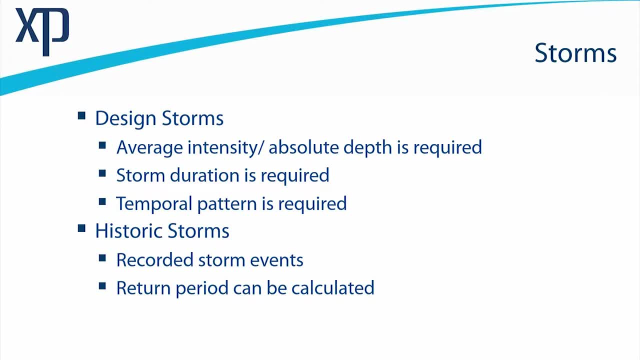 I need to assess a range of storm durations. This sort of approach, this design storm approach, is not an equivalent to the rational method. I'll talk a bit about the rational method shortly. but it's not a situation of modelling simply one storm duration. 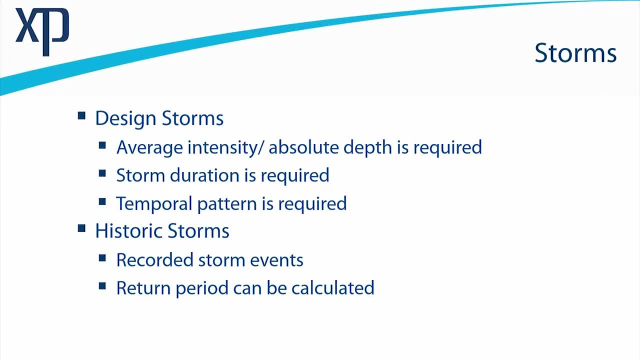 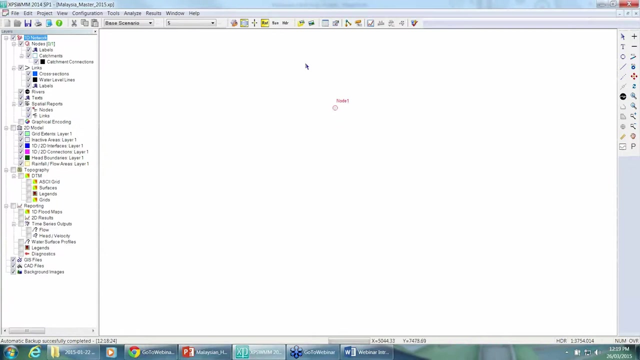 We'd need to assess a number of durations, And the temporal patterns do come from the MSMA2 documentation, which is a great reference manual for the Malaysian region, and I hope that everyone either has a copy or is familiar with that document. I'm going to go into the software and I'll show you inside our software how the software 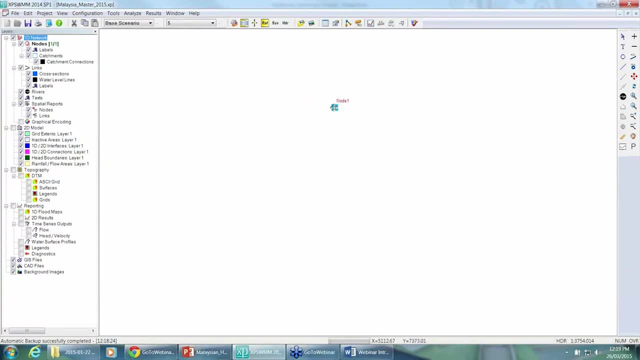 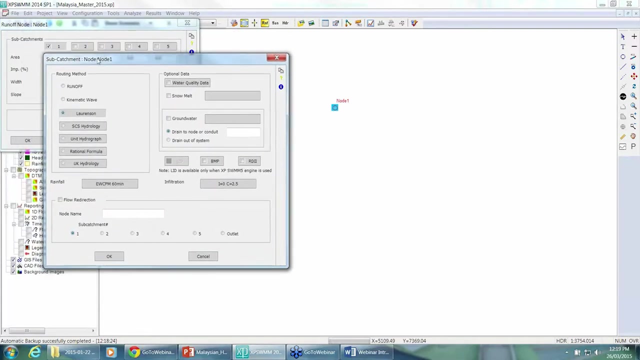 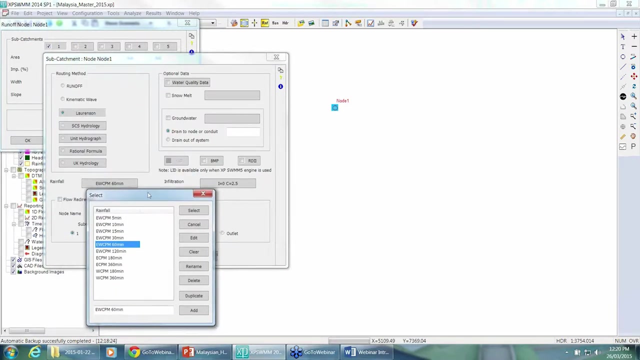 deals with Malaysian information. So on this node 1, I'm just using this as a representative catchment And I have just applied a simple 1 hectare area to the catchment. But inside the interface I have some rainfall information and a variety of different locations. 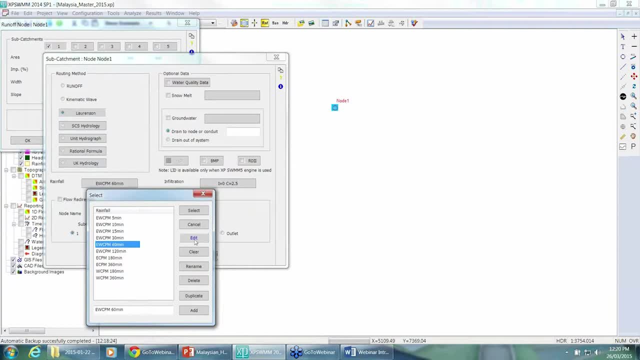 We can create locations anywhere across Malaysia, but if I just create a new one, I'll call this JPS. So I'll call this JPS, And that's that, And that's that, And that's that, That's that. 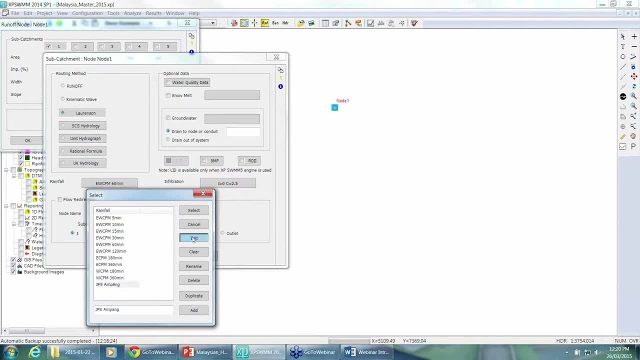 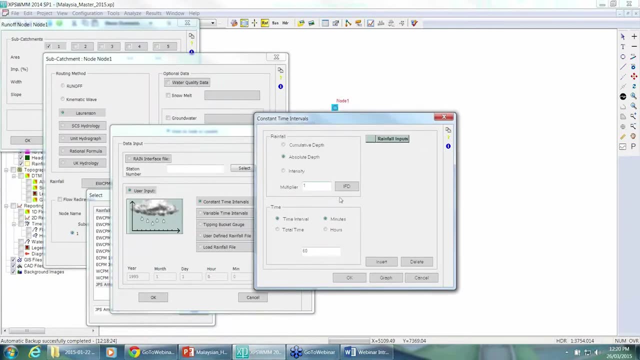 And that's that, And that's that And I'm going to hit to add. I'll edit this, Go into this particular dialogue box And I have an IFD calculator- This is specific for Malaysia- And this IFD button I can select the type of ARI for the study. 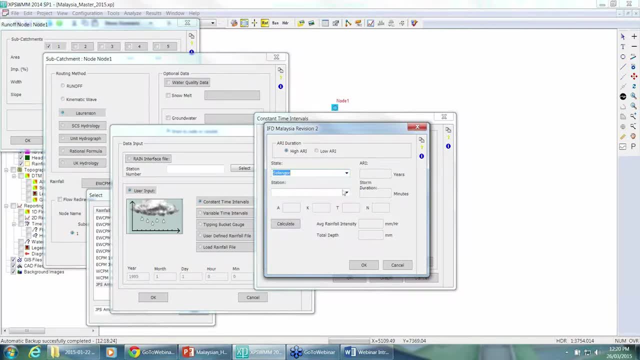 Select my location. So if I were to go to Selangor, I can select JPS Ampang, Nominate a ARI and a duration event and press the Calculate button and that will define the average rainfall intensity or depth of rainfall, and it's exactly the same, because it's 60 minutes in this example. 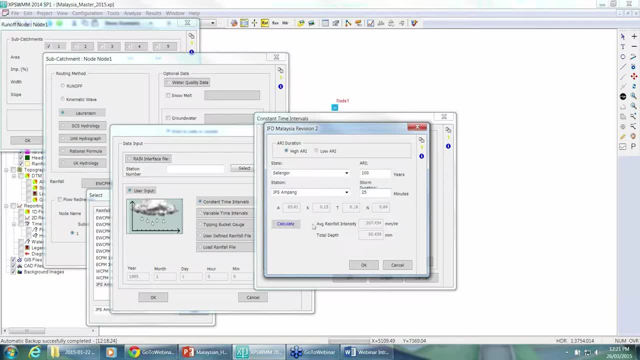 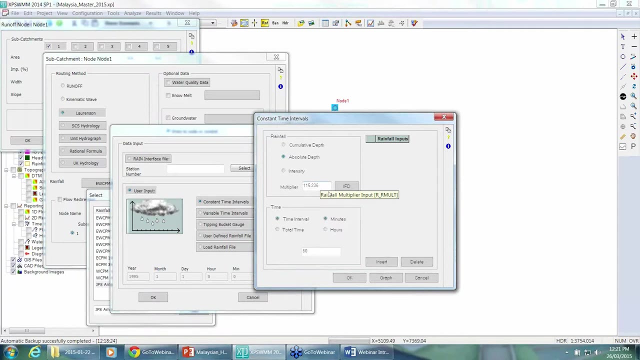 But if I were to change this, I could recalculate for 25 minutes and it would give me that variant detail. So that's a very useful utility for our Malaysian clients. I'll just change that back to 60 for this example And that information gets back populated here and we would just 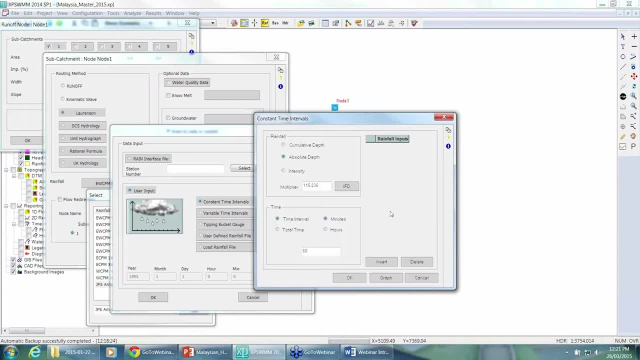 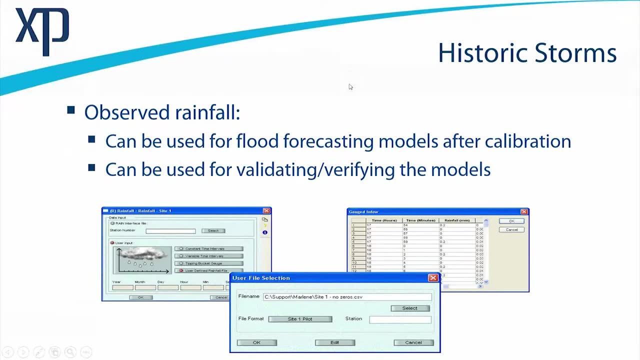 apply the temporal pattern for that 60 minute storm from the MSMA to guidelines and I'll show you one of those a little later on Back into the slide. So historic storms I can take observed rainfall data and if you can get information from the Bureau of Meteorology. 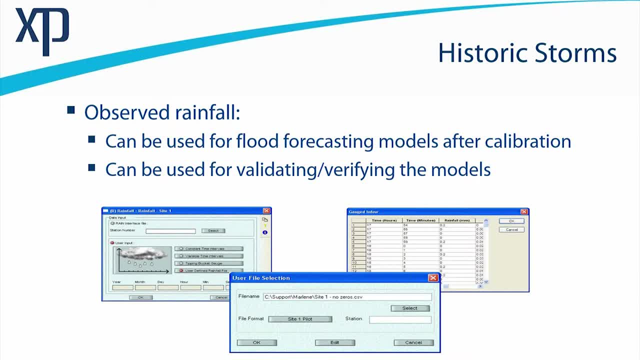 or your local authorities in Malaysia. we can take this information to use it for flood forecasting purposes. thorough calibration, and once you've undertaken a calibration, you definitely want to validate or verify that model with another historic storm event. And one question that was posed to me recently: 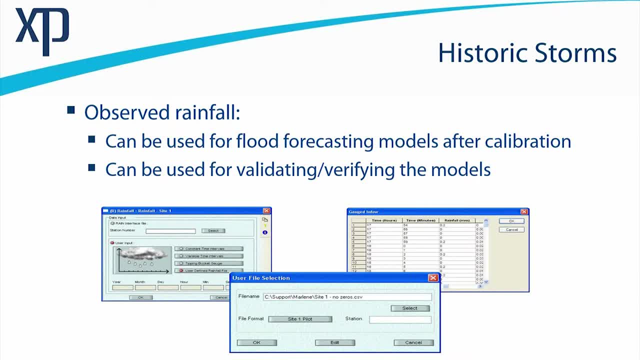 One question that was posed to me recently was from the Malaysian region- was what is the accuracy of the rainfall data sets that we need to have to undertake these historic studies? We definitely need sub-daily time steps. Ideally, you would want to obtain the 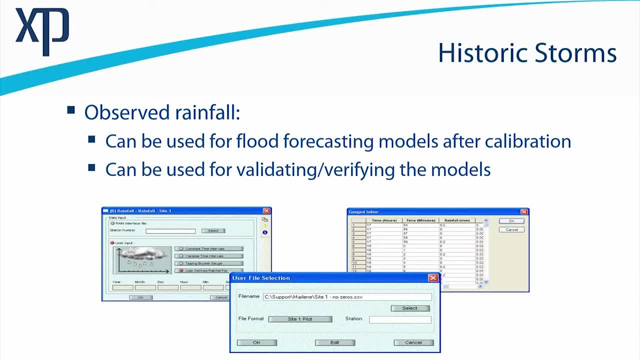 raw rainfall data to allow an appropriate study to be undertaken. Taking daily values simply distorts your ability to analyse a catchment because you'll have to assume the rainfall occurred consistently over the day, whereas we know that rainfall spikes in sometimes very brief periods, either 5 or 30 minute periods. So daily historic data. 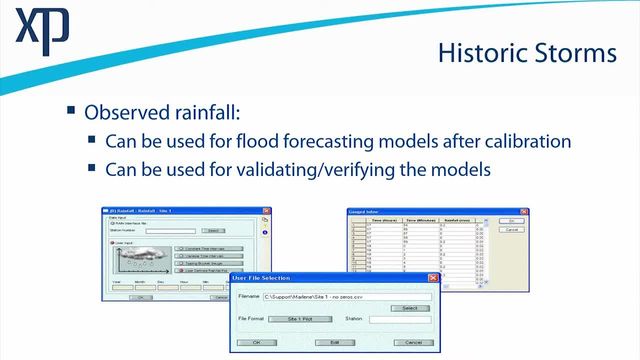 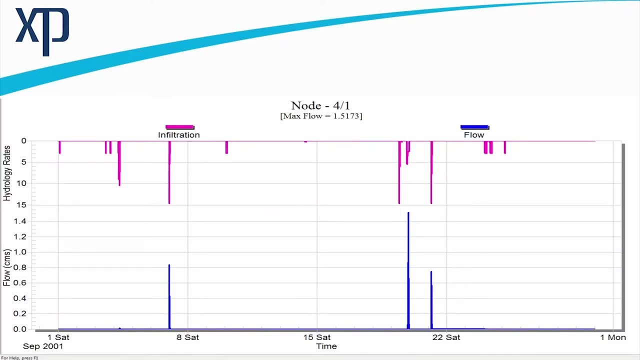 is inadequate. and if you're able to procure sub-daily values or again that raw information, when did the rain gauge tell us that it received a millimetre of rain? that would be a much better data set to analyse. We can feed in those rainfall values. 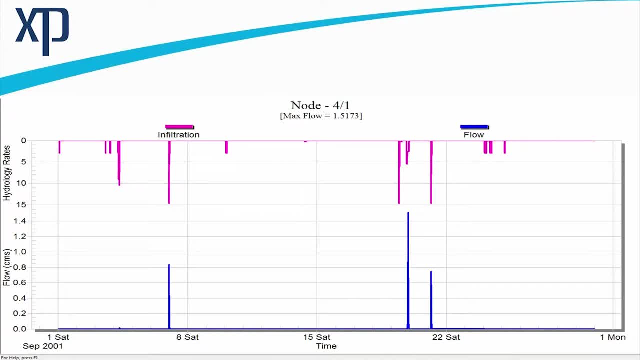 We can apply infiltration procedures to that to define discharge from our catchments. And so what I've done here with a real rainfall set is applied, some ongoing losses- and we can see that because of the potential for catchment infiltration, we don't actually have any runoff in response to these small events. When we get into these larger events, 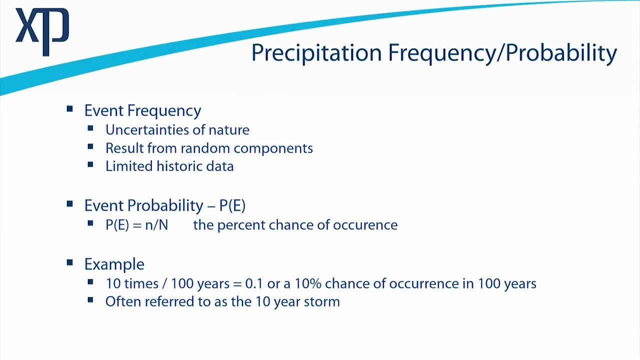 we see spikes in our runoff record. So obviously if, in the absence of design information- which fortunately Malaysia actually does have a pretty good data set of you, could look at some statistics to back derive your design events, looking at the probabilities of events occurring over time by doing an assessment of your rainfall records. But again, the fact, 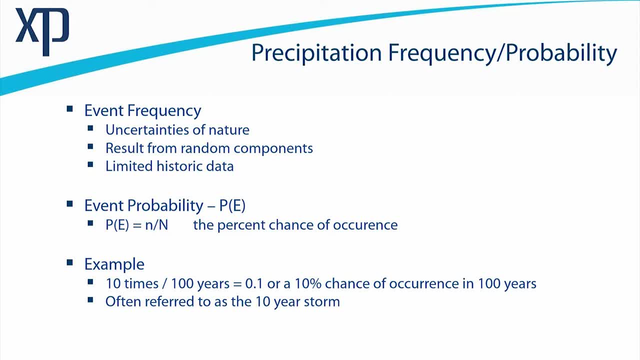 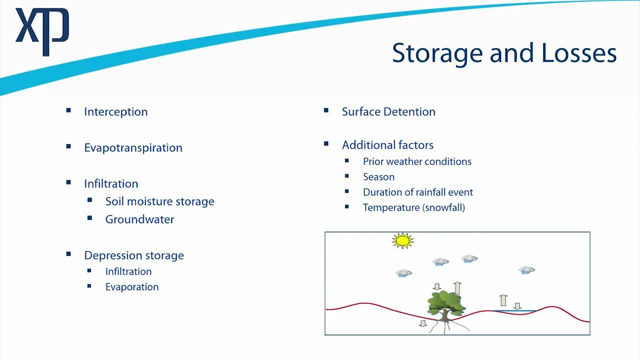 that we have design data in Malaysia makes this not a common task. Just quickly back on storage and losses. Another loss that days sometimes accounted for is interception. Now, interception is most regularly considered in an urban context to be rainwater harvesting, So a rainwater tank. 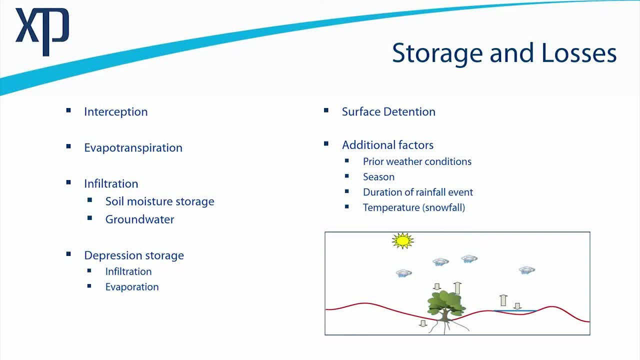 is actually an interception device. It takes that rainfall from your roof areas, stores it and hopefully it's used for beneficial purposes post a storm event, be that for landscape irrigation, toilet flushing, lawn mowing, toilet flushing or, potentially, laundry washing. evapotranspiration from the surface plus your 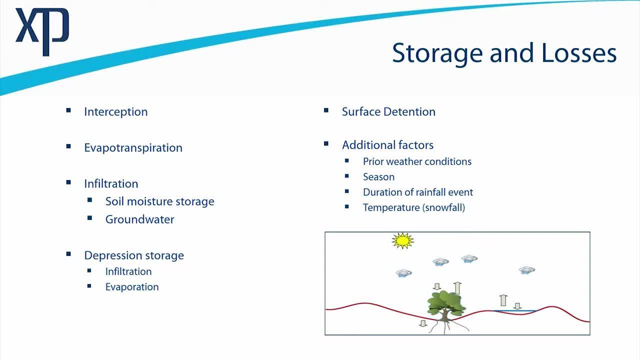 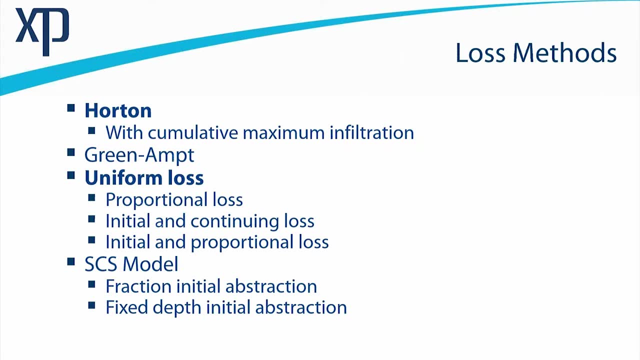 vegetation again. infiltration we spoke about before, But these factors all need to be considered in your hydrologic calculations Inside our software. we actually have four dominant loss methods. However, for the Malaysian context, only two of those really stand out as being appropriate. 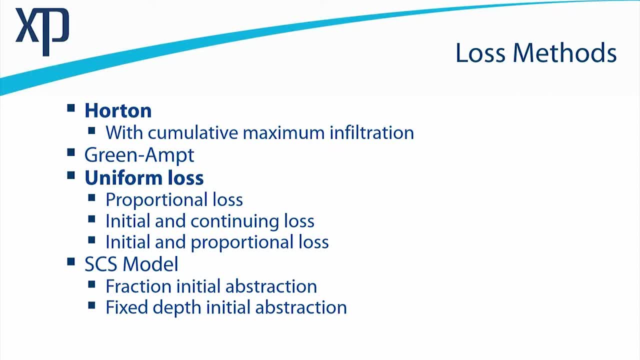 as per your guidelines. The first of those is Horton's method, and it can be adapted to be a continuous loss method if you were trying to run a long duration time series, for example, years worth of rainfall under historic analysis, or uniform losses, which are most commonly applied for design. 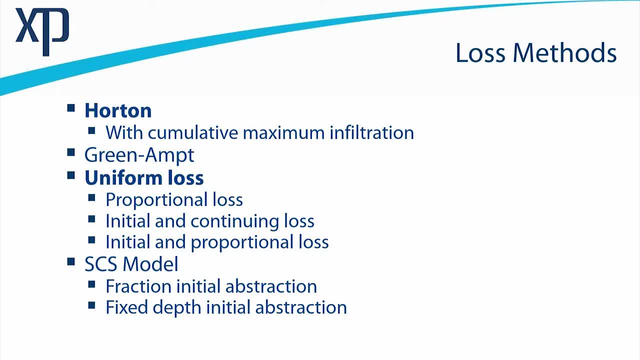 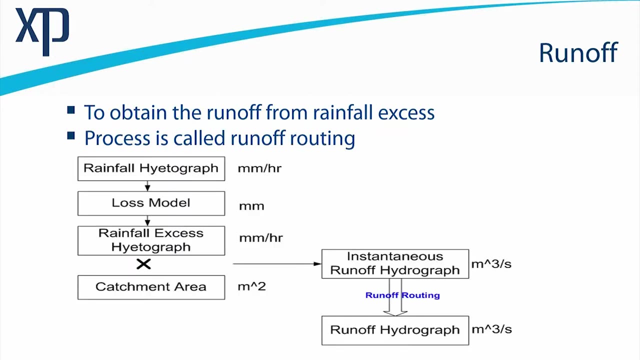 storm modelling. The common option out of the three uniform loss types is the initial and continuing loss method, But we do have green, AMT and the Soil Conservation Service methods which are used around different parts of the world, particularly America. In defining or deriving our runoff, we run through a process of taking the rainfall hydrograph. 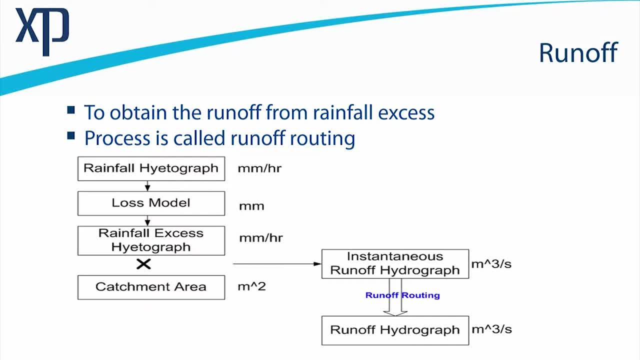 which is either the design storm temporal pattern from the MSMA 2 guidelines, multiplying that by the IFD value that we may have obtained from the calculator calculator inside XP Swim. Subtract that loss model. that initial continuing loss would be the most appropriate way. Define an excess hydrograph. Multiply that by our catchment. 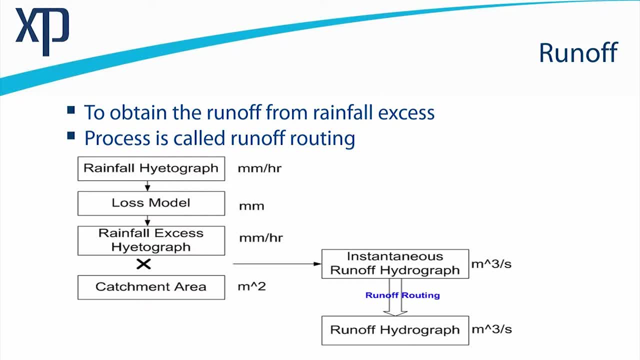 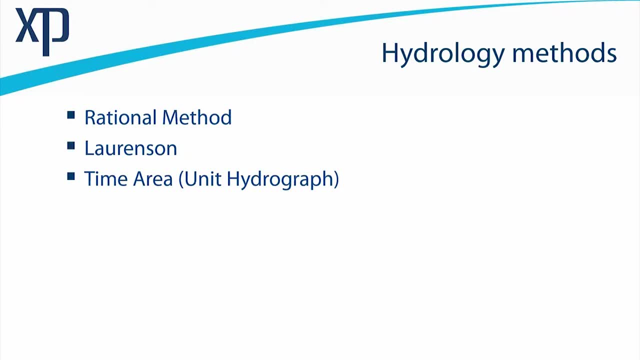 area to generate our hydrograph for assessment. Now, inside the software we actually have about 23 or 24 different hydrology methods, But the three that do stand out for the Malaysian context are the rational method, Lawrenson's method, which is referred to by a number of 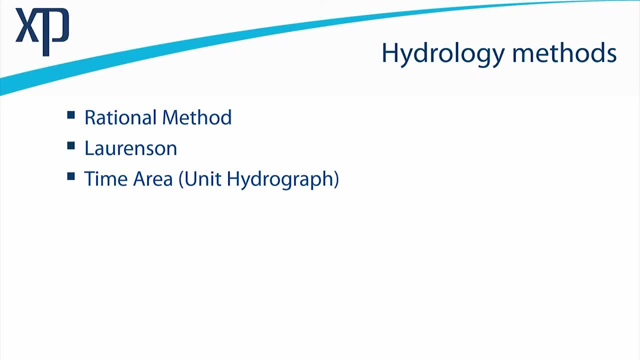 people in the industry as rafts, but the actual equations behind that is Lawrenson's method and also time area. From my perspective, I would always pick Lawrenson's method. It is by far the more advanced method of these three and it is definitely one of the recommended. 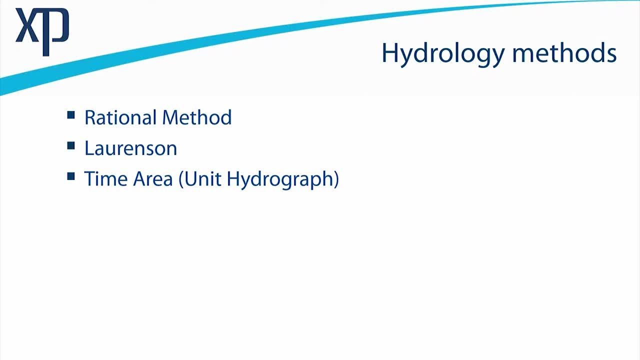 methods out of the MSMA2 guidelines for application in Malaysia. Now the rational method is the one that is used in most of the MSMA2 applications. The rational method is the one that is used in most of the MSMA2 applications. Now the rational. 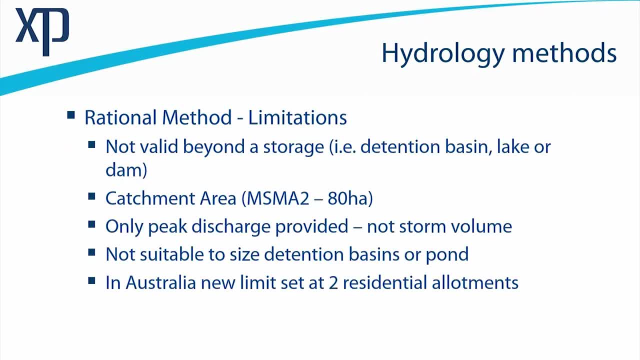 method is the one that is used in most of the MSMA2 applications. Now, the rational method is the one that is used in most of the MSMA2 applications. Now, the rational method does have a number of limitations, and that's something that people do need to be aware of. from a 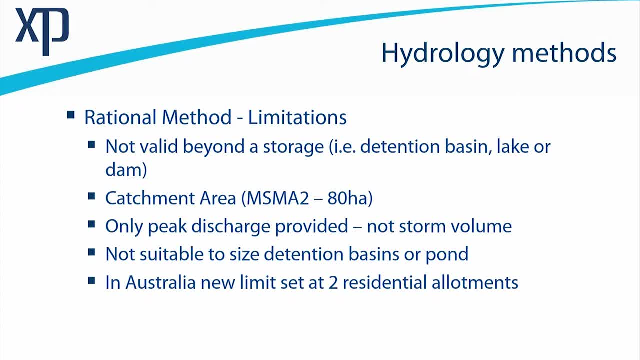 hydrology perspective, And that is that it's not really valid beyond any storage system, whether that be a detention basin, a lake or a dam, And so that can be quite a difficult element to factor in, And if you're working in new development areas that have large scale. 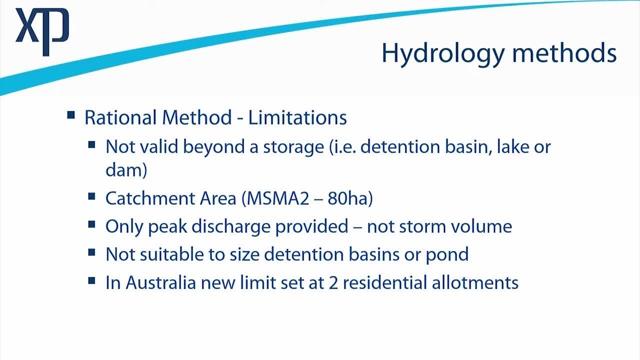 rainwater harvesting systems, that too would be another reason to factor in, And if you're working in new development areas that have large scale rainwater harvesting systems, that too would be another reason to factor in, And so that can be quite a difficult element to factor in, And so that could be quite a difficult element to factor in, And so that could be quite a difficult element to factor in, And so that could be quite a difficult element to factor in, And some of theㅠㅠ. 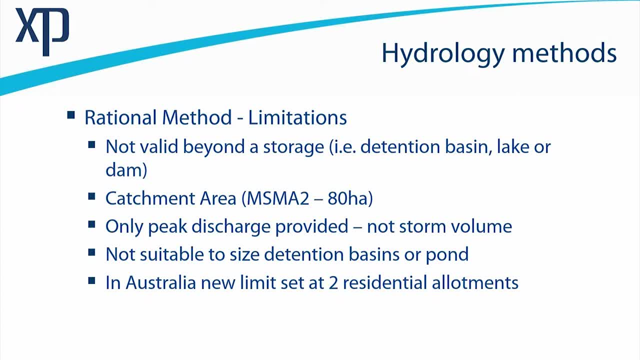 include the nah. The other parts of the world do have some high limits than that. However, here in Australia, our main storm water guideline is being updated and it will limit engineers in this region of the world to only allow you to model 2 residential allotments using the rational method. Now, that's a very small area that. 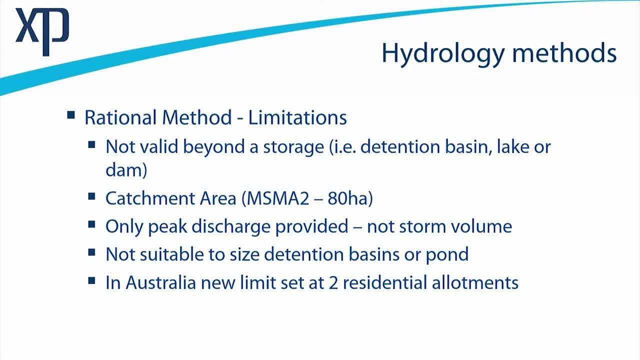 could be 800 square metres. So I'm not talking in hectares anymore, we're talking in hundreds of square metres as a limit to the rational method. So that has some far reaching consequences. Of course, the key limitation is it only tells us a peak discharge rate based on the concept. 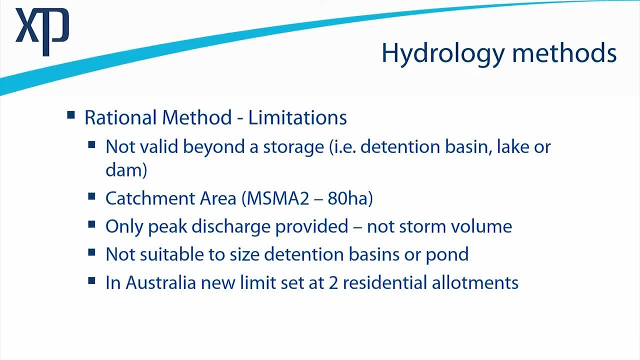 of the time of concentration, which means that it's not suitable to size detention systems. Now there are some equations to try and force the application of the rational method to size storage devices, but they're by no means rigorous relative to the data that we have. 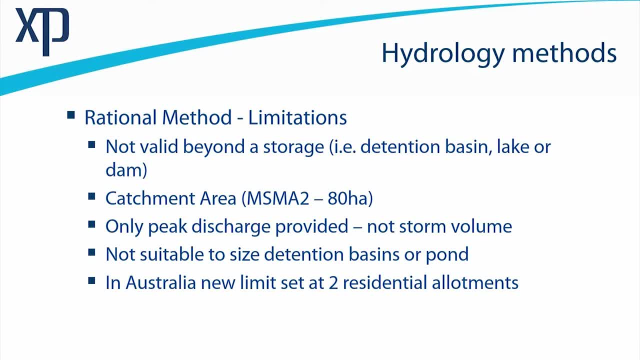 available in terms of our design, storm information or our ability to undertake calculations very rapidly inside computer packages such as XP-SWIM. Some key parameters that we need to deal with, in order of importance: 1. The size of the storage devices. 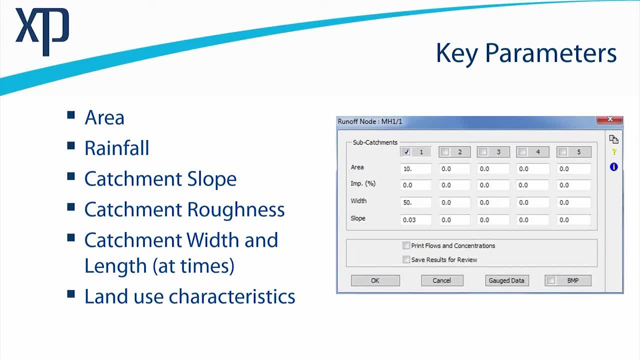 2. The size of the storage devices. 3. The size of the storage devices. 4. The size of the storage devices. 5. The catchment area. That is the most dominant parameter that we need to play with. 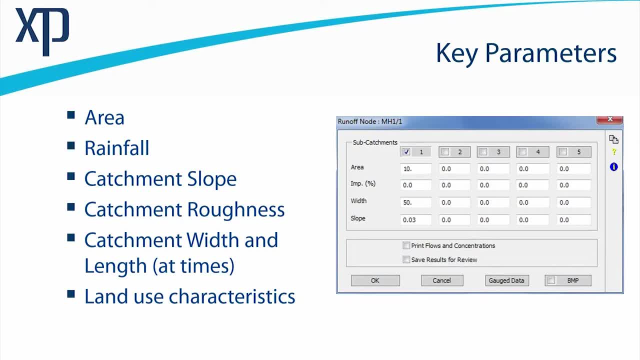 6. The rainfall, Again using the temporal patterns and the IFD information, We have other parameters that then support Lawrenson's method in particular, which are: catchment slope, the catchment roughness- Some methods, but not Lawrenson's method. 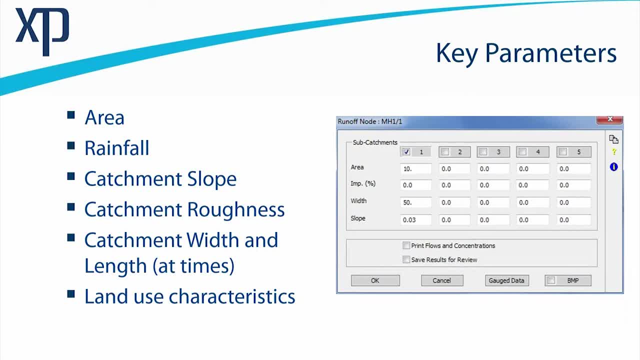 use catchment width or length. So if you were trying to undertake a Bransby-Williams style calculation to derive a time of concentration for a catchment, if you felt that was appropriate for you, then by all means you would definitely need the catchment width in that equation. So from 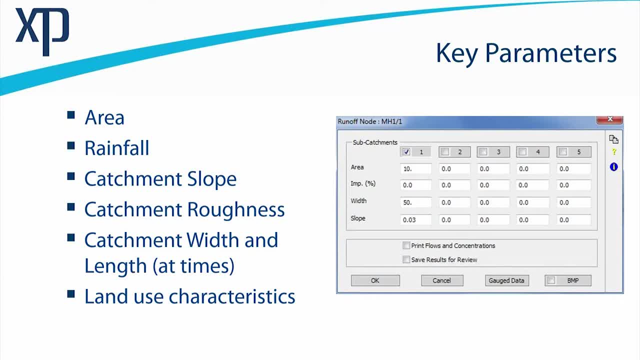 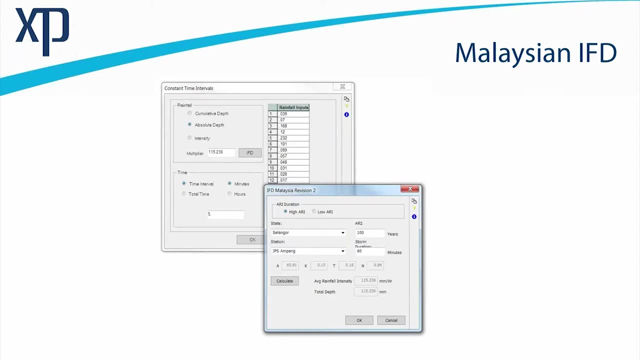 the total area and the width, we can imply the length, And then an understanding of the land use characteristics which helps us define our infiltration or our losses. That's just a quick review back on that IFD calculator, same location that JPS Umpung. 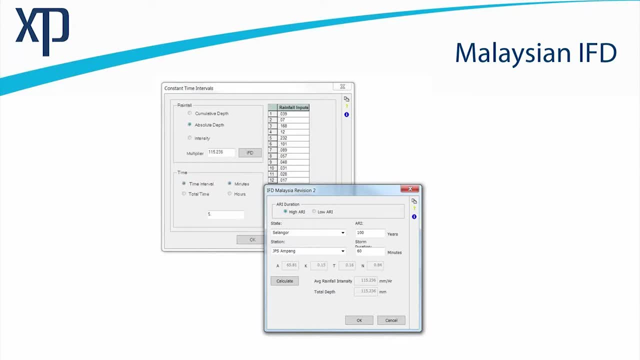 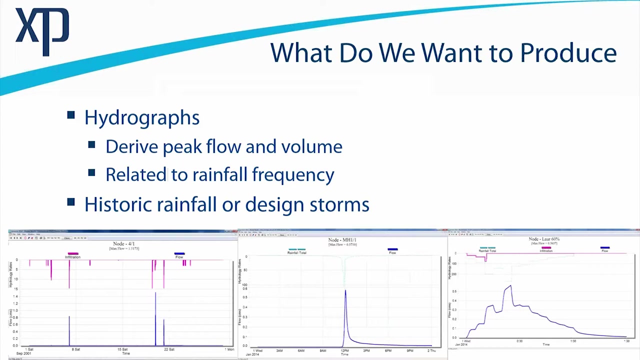 which shows with a temporal pattern applied- that's, the 60 minute pattern- and how that would be applied to the software. And so, from all of that background information, what is it that we're trying to achieve? Why are we interested in running these calculations? And of course, it's to derive these peak flows. 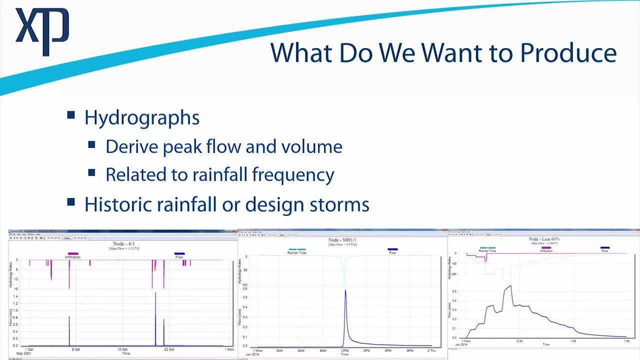 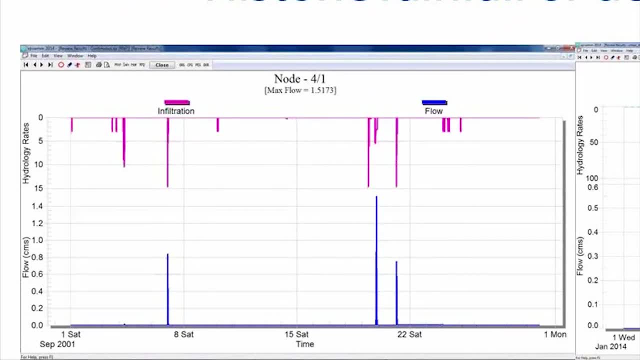 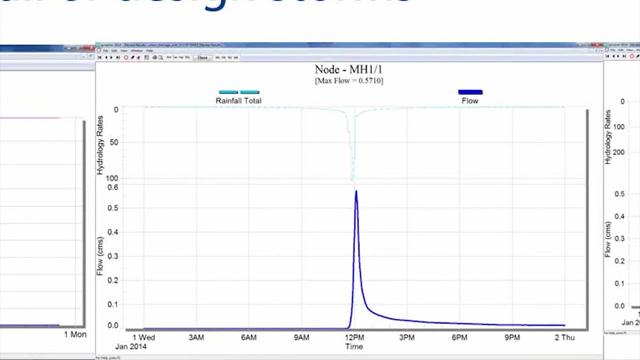 and volumes relative to our rainfall input. And so these are three shots that I have at the bottom of the screen here. One shows that long duration analysis, that's a month's worth of rainfall, versus a specific rainfall event in the middle or a design storm on the right hand side, And each have 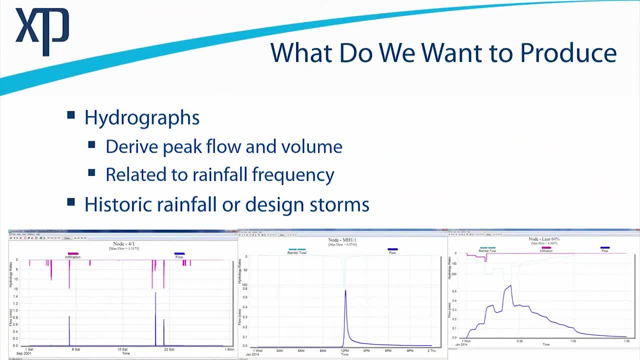 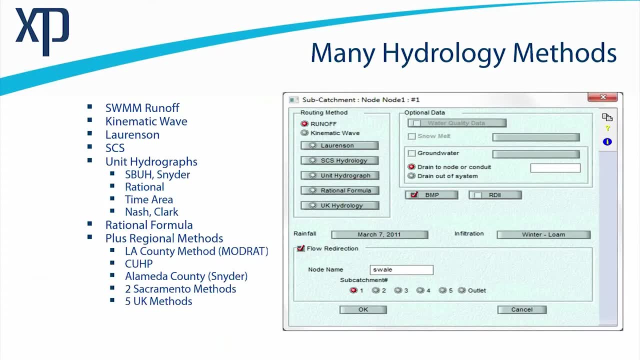 distinctly different approaches to them, but the important thing is to be able to analyse all of these if and as required. Just for background information, we do have again. there's many hydrology methods that we're going to be talking about in the next few minutes, but we're going to be talking. 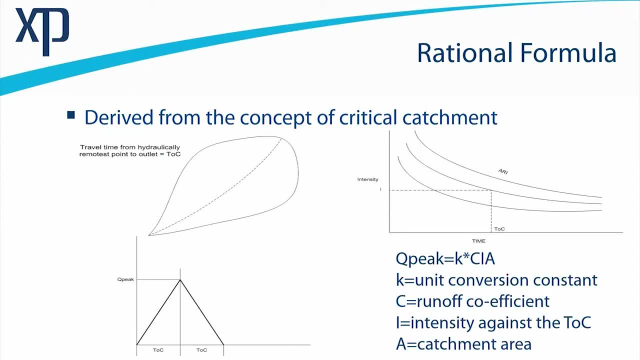 about the rational methods in addition to those three that I talked about before. But just focusing on the rational method quickly, it is derived based on this concept of a critical time of concentration and most people are very happy with it and are understanding it. 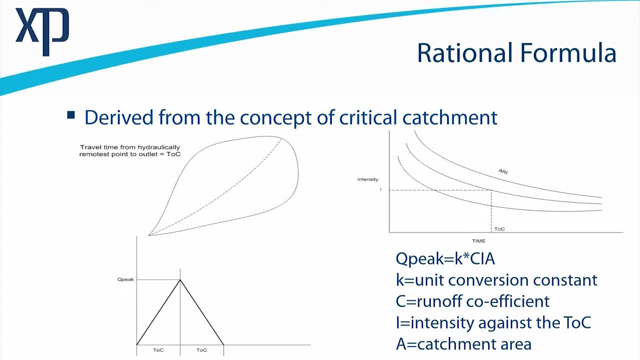 I think it's a very good rule of thumb, but it is by no means the be-all and end-all of a hydrology calculation set And by no means would I expect that to be the case. So I think that's pretty clear and I think that's going to be good for you. 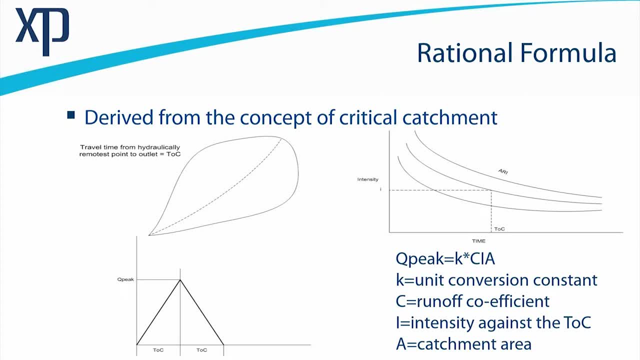 Now, as an example, you can see that the hydrology is based on an image over here, and that's the point we're looking at. You can see the rapidly changing image over here, and the amount of energy that's being deployed on the surface of the water is going to be one of the most important things to 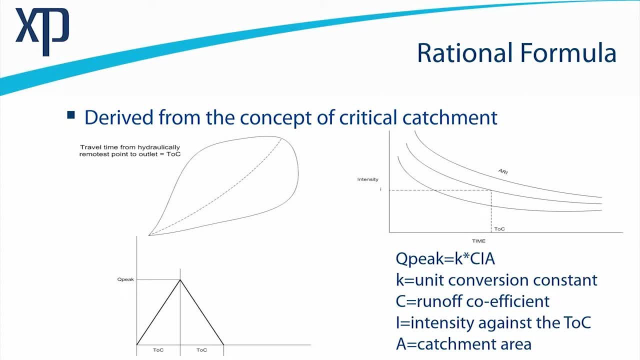 do. Now, that's not a terrifying thing to look at. It's actually quite clear to see and again, it's important to, as I said, give you a the correct answer. But that's more to look at than anything else that's going to affect the performance of. 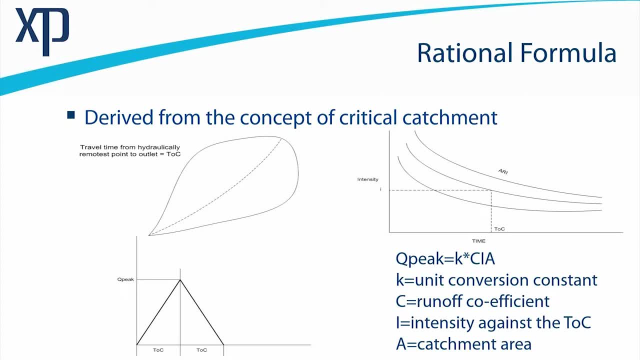 your water policy, which is how the water is being used. So over here I don't want to stress, but at this point in time I will point out a couple of things that are good to look at. does a river system perform in the real world versus our calculations? Now you could try. 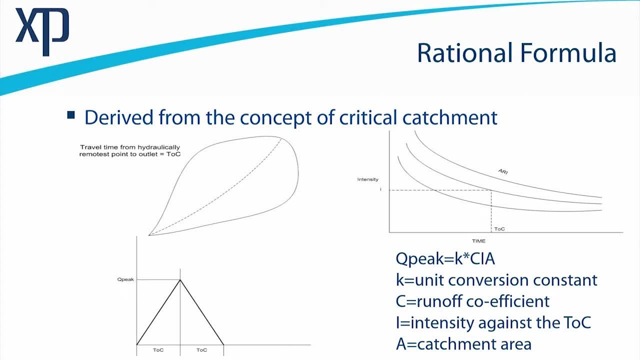 and calibrate the rational method to the real world. you could also try and calibrate Lawrenson's method to the real world, and your approach would be slightly different in both examples, but with the ability to get more information out of a hydrology method, which would give. 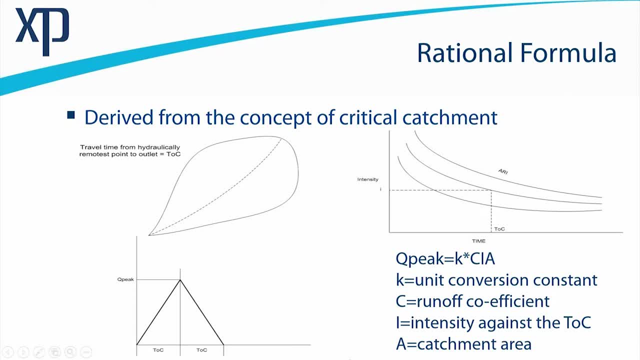 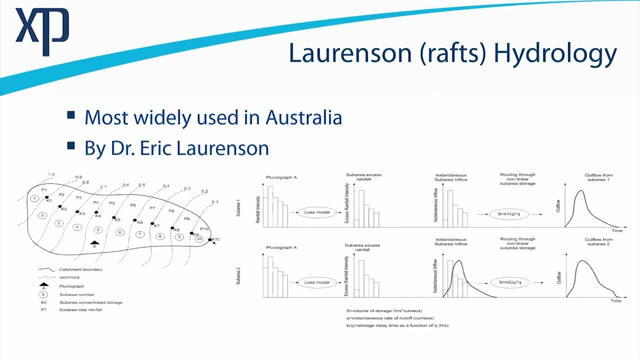 you not only just the peak discharge rate in the river system but also the total volume that contributed behind that peak flow rate. This Lawrenson's or Raff's hydrology is very common here in Australia but it is also very common in Malaysia, developed by Dr Eric Lawrenson, and it runs on this principle. where any individual 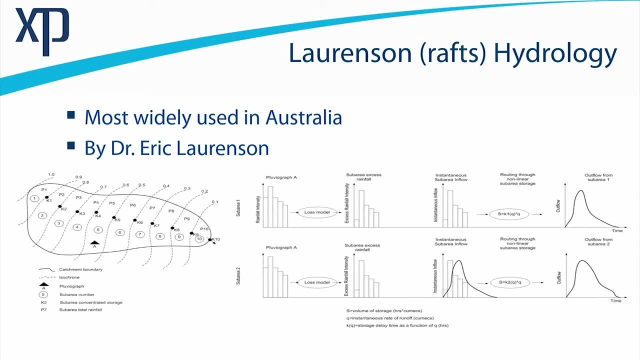 catchment is broken up into 10 sub-elements, routed internally and based on a storage equation, and that storage equation is a function of catchment area, the roughness of the catchment and urbanisation factor. so that's a function of the fraction, impervious and roughness details. 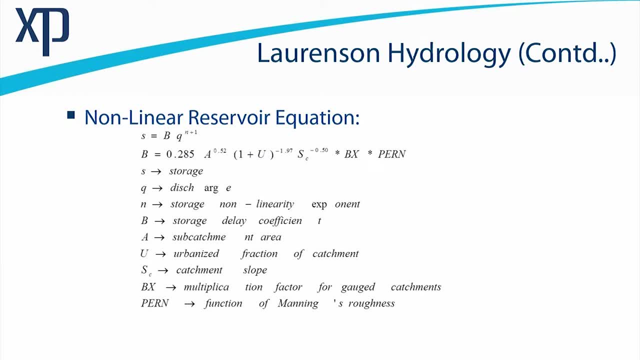 And so this is the core equation, where storage is a function of this B parameter, and B has a bigger equation below it, also known by flow, and then a non-linear flow equation. It's a linear exponent, and so the reason we need to use a program for this is because 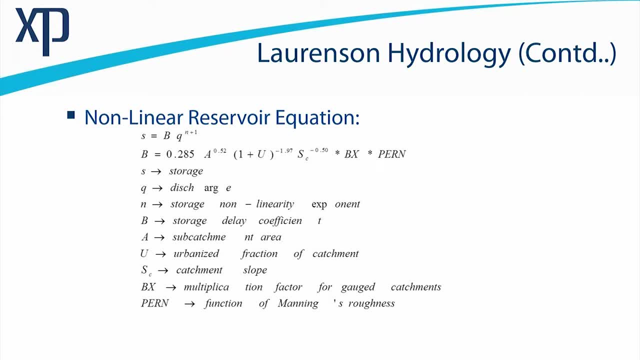 the first time step. we don't know S and we also do not know Q, and so we need to apply an iterative solution to the system to derive our results. But the B parameter, the B equation, is actually well defined. it's all based on physical parameters. 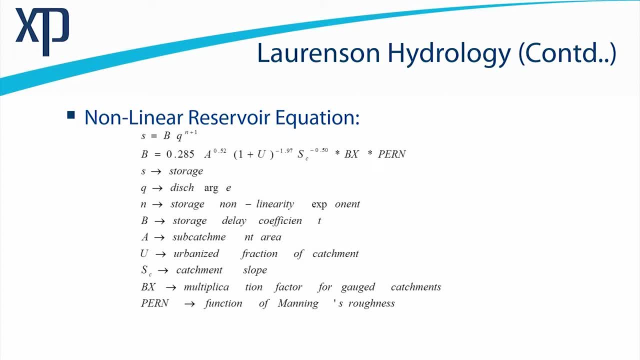 although we do have a BX value in the back there which is a multiplication factor for gauged catchments, if we need to make a slight adjustment to factor in some of the parameters that occur in the real world that can't be factored into what is relatively a simple 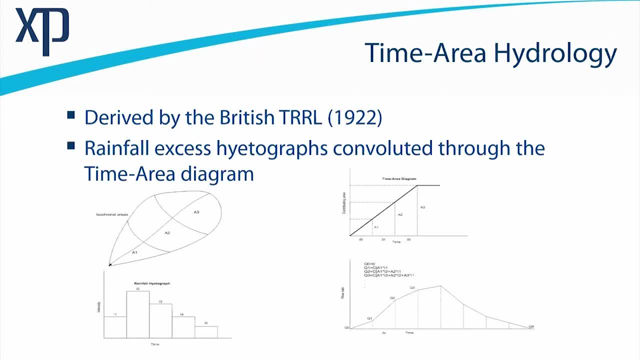 equation Time area is another popular method I understand in Malaysia, although again, I would likely not personally try and apply this in Malaysia. I think it has a few limitations on it in terms of larger catchments, But also not necessarily flexible enough relative to the demands for detention basin calculations. 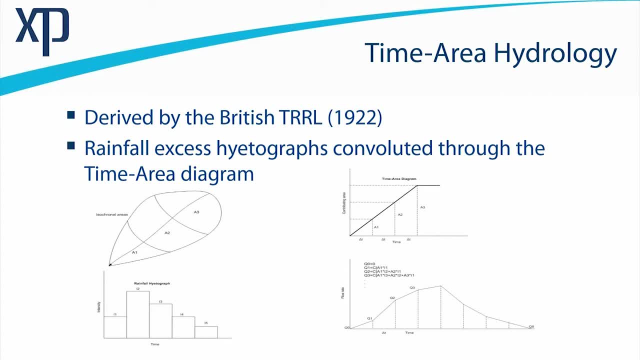 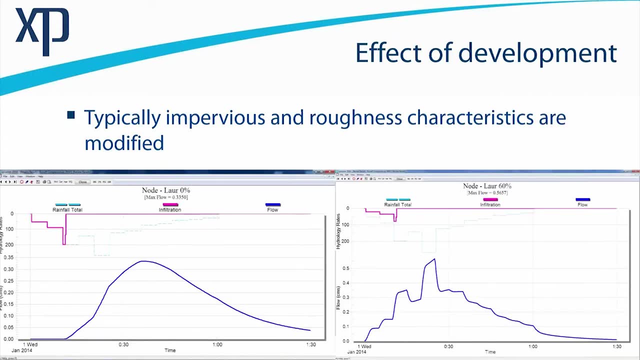 So running a more rigorous hydrograph method like Lawrenson's method is not only quicker but makes assessment more rigorous. When we take any given site and start with a low or limited impervious component and then compare that to a fully developed site, we get these substantial changes in the shape. 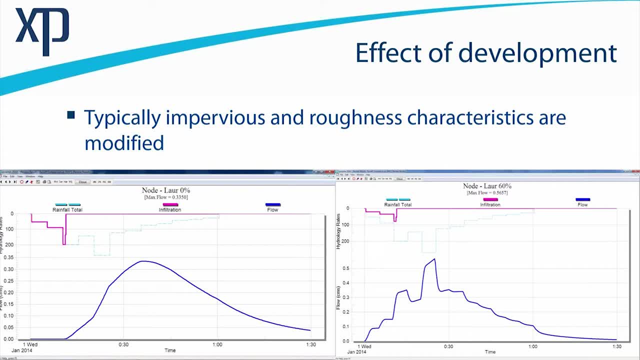 of our hydrographs. So the curve on the left hand side: there is a nice smooth curve from a zero impervious site and the curve on the right hand side is showing a 60% impervious site using Lawrenson's method against a temporal pattern, a design storm And the area underneath. 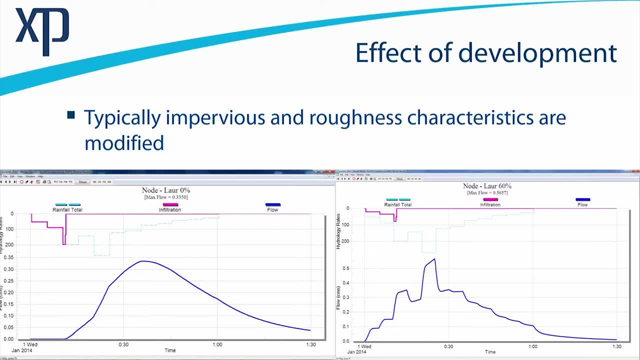 The area underneath the curve on the right hand side is greater than the area underneath the curve on the left hand side, so we've got more water as well, not only a much bigger peak discharge rate, so going from just shy of 350 litres per second to up near 550 litres. 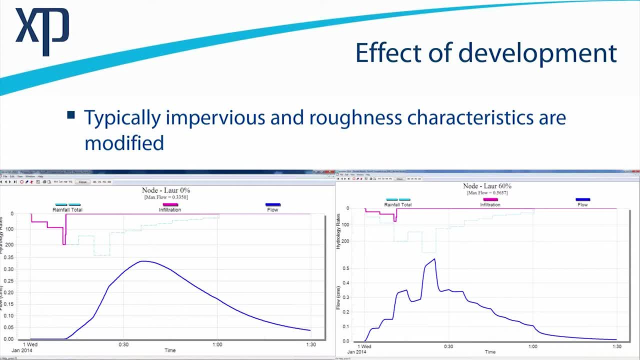 per second in response to development And hydraulically. you would then need to look at potential solutions to try and mitigate that increasing discharge and at times, if you have a volume controlled catchment, you may need to look at clever ways to store that water and hopefully limit it in getting down. 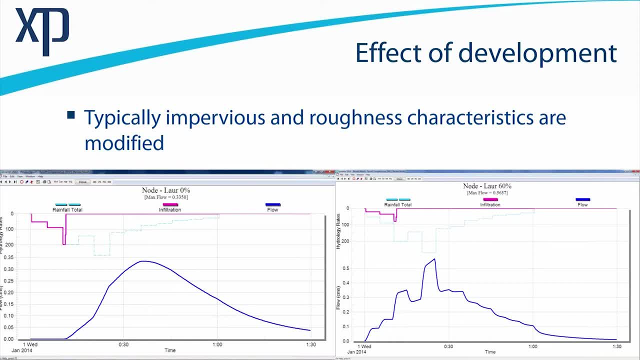 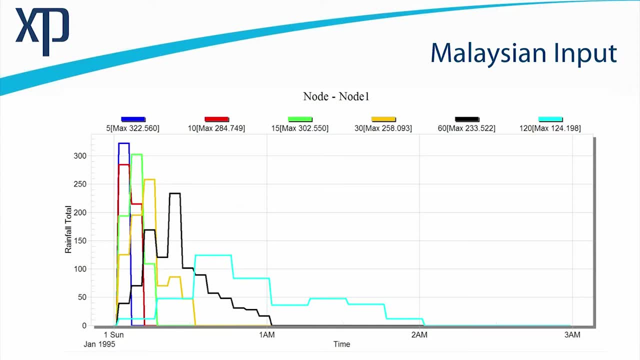 to the river system if you have again a volume controlled river system. So I've just taken some snapshot of the Malaysian temporal patterns and so this shows a range of the patterns from the 5 minute through to the 120 minute. This does come from. 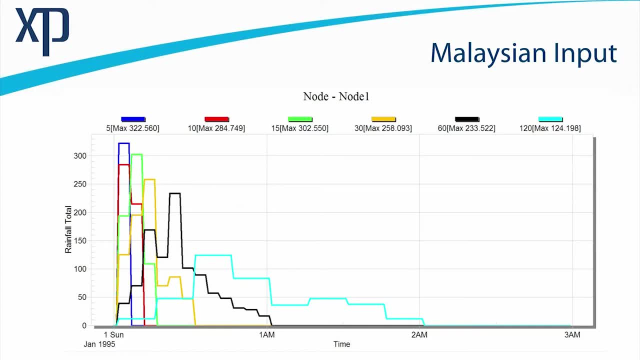 the MSMA2 guidelines. a bit hard to see with the overlap, but you'll get a perception. This is the temporal patterns multiplied by their respective IFD values to put them at a scale. And when we apply these with Lawrence's method inside the software we can generate these. 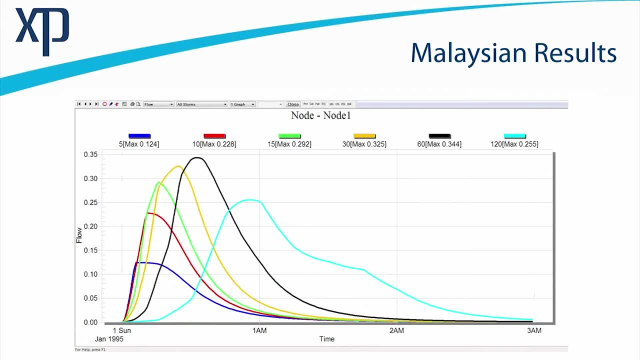 discharge curves and for a simple catchment. I think this is my 1 hectare example for a undeveloped catchment, So 0% impervious catchment. my critical storm is actually the 60 minute event. Now if we were to convert this to a developed case, then I would expect to see that possibly. 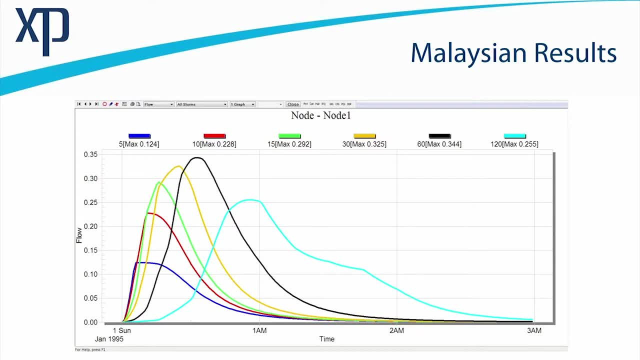 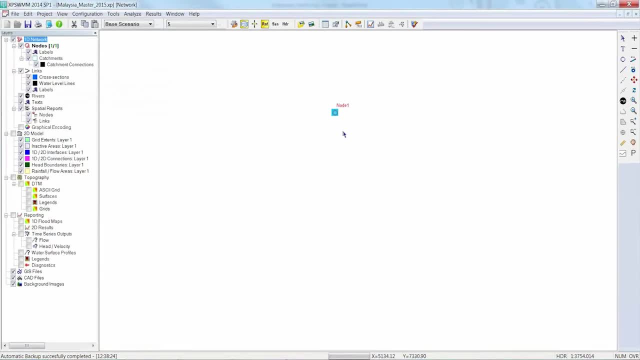 the 15 minute or maybe the 30 minute pattern might actually be the dominant pattern in response to the change in fraction. impervious. I'll just jump back to the software just to give you an indication of how long it takes to run this model. 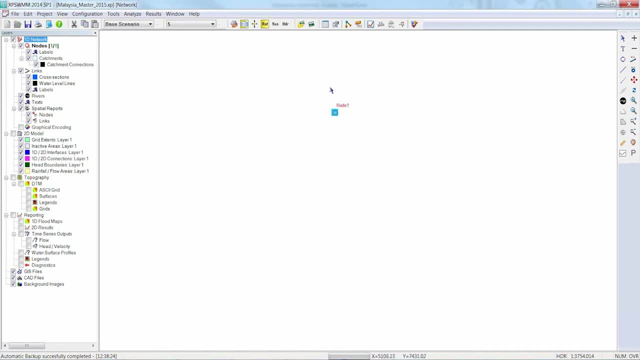 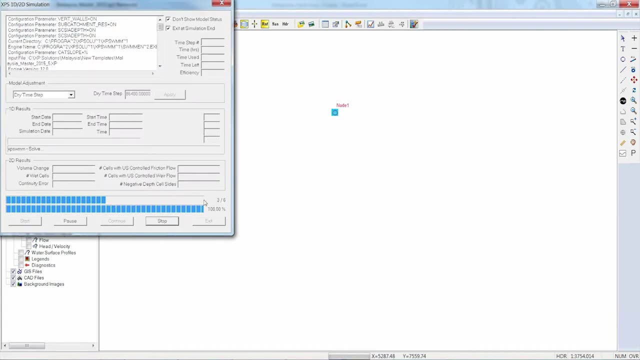 So obviously it's not a simple model only, It's a very simple model. It's very simple. I'll just show you the one node. at the moment, If I hit solve, I'm running these 6 storms and it is as quick as that. 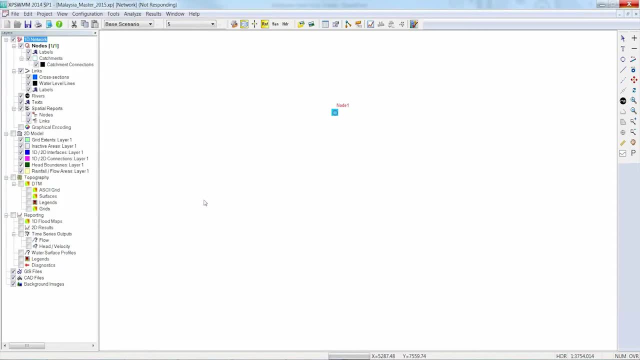 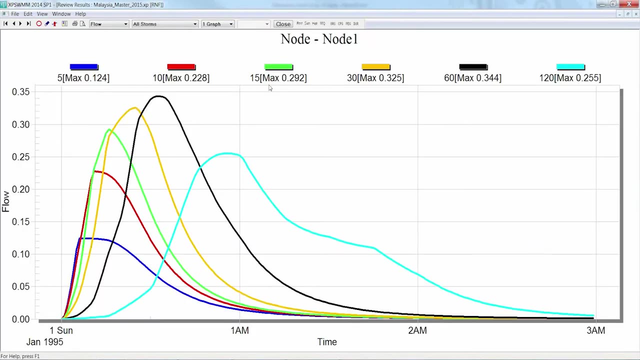 For me to prepare this off limited information. it takes me almost no time to obtain some rapid results. It's that same set of results from the software. And not only can we obtain for these multiple storms, peak discharge, but I can look at rainfall. 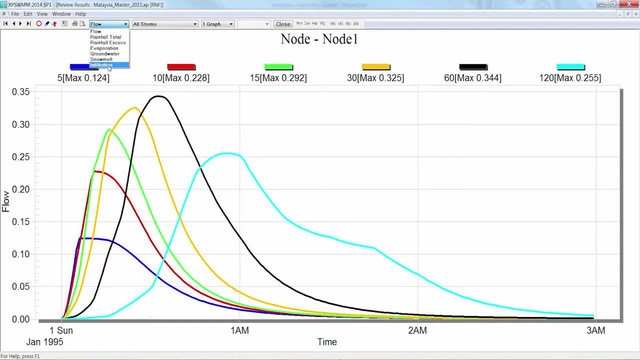 totals The impacts of infiltration and other parameters, and I can also isolate down and just look at one storm, if I wish For reporting purposes. it's very important to be able to get this information across to not only our clients as consultants or interested individuals at a state government. 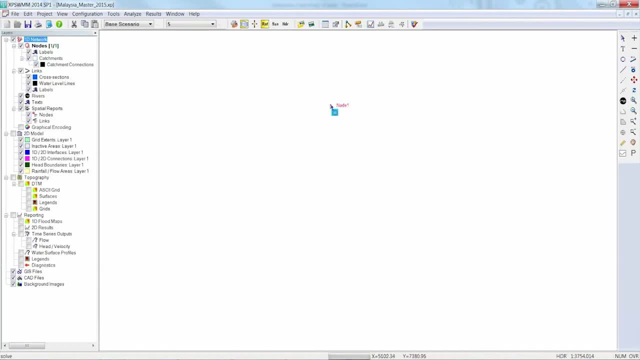 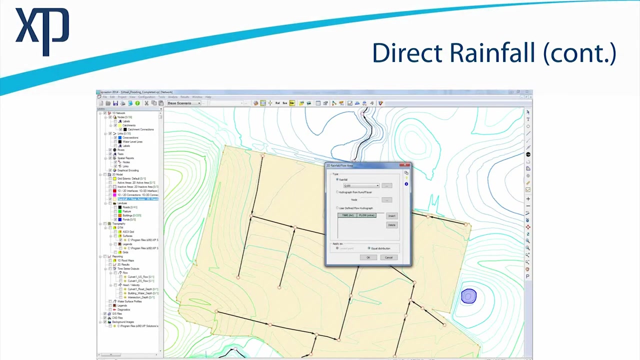 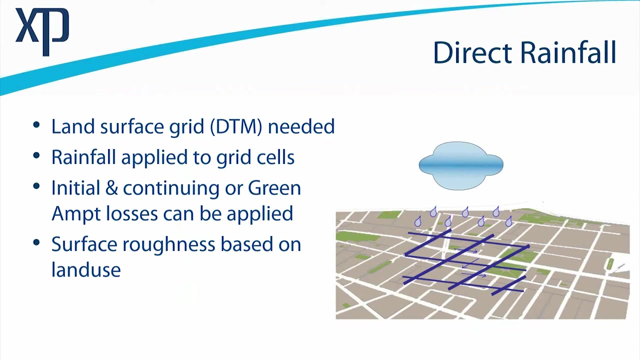 or assessment level, So very quick to model inside our interface with limited information. What is becoming really popular In certain parts of the world is this concept of direct rainfall, and that concept relies on a 2D model rather than a .1D model like that simple one node that I showed. a second: 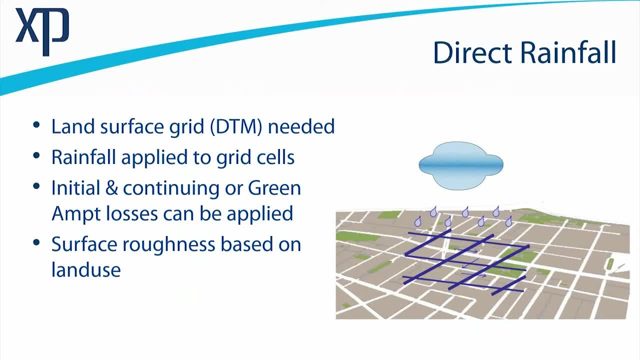 ago. It means we need to have good service information and unfortunately I'm aware that that service data is at times limited in the Malaysian region, but over time no doubt the capture of information we get in the formal infrastructure will improve. Slide 003 – Comparing Web-based survey metrics with LIDAR measured data. 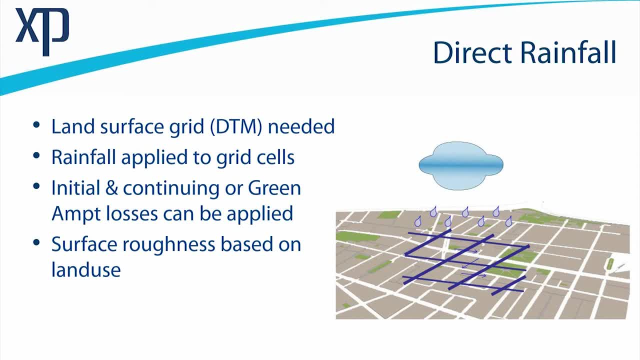 Slide 003 – Comparing Web-based survey metrics with LIDAR measured data. Slide 004 – Comparing Web-based survey metrics with LIDAR measured data. low points and accumulate as it would, hopefully, in the real world. There are some limits to it in that you do need to have a relatively fine terrain data. 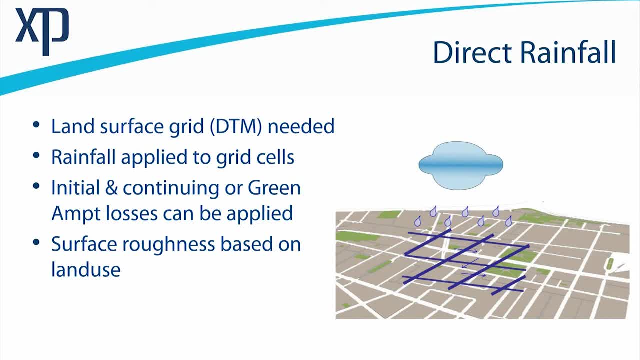 set. That's our biggest limitation in the short term. Secondarily, you need to understand your land use and then also the impact of surface roughness elements. And those surface roughness elements could be in the form of a building, because typically when we have our aerial survey, we remove or filter out buildings from the surface and 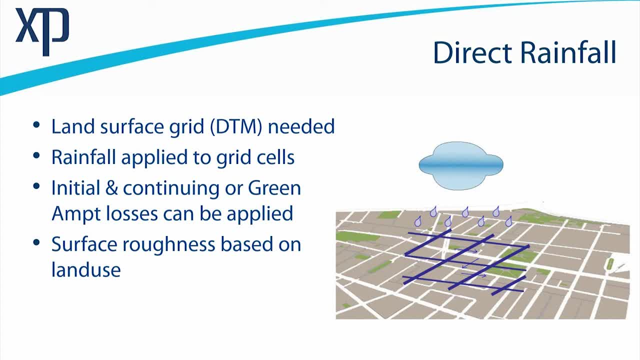 so water would inherently try and flow through where a building is. and, of course, hopefully, your buildings are generally impervious at their lower components. if they have a concrete slab or if they're an elevated building, well, maybe that's not so important if they're a 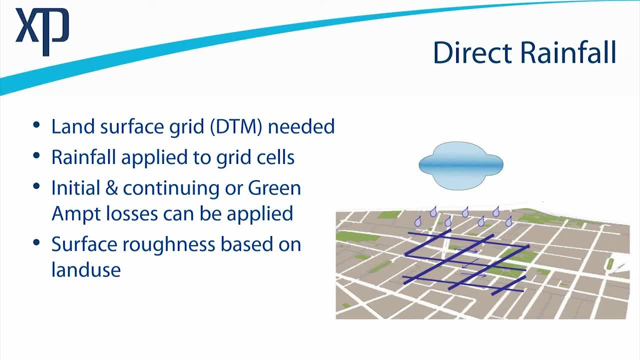 pole home. But understanding the impact of buildings and also fences, particularly block work fences, becomes a difficulty for these models. But here in Australia and America and other parts of Europe, direct rainfall is really taking off to undertake very large area studies respectively quickly.